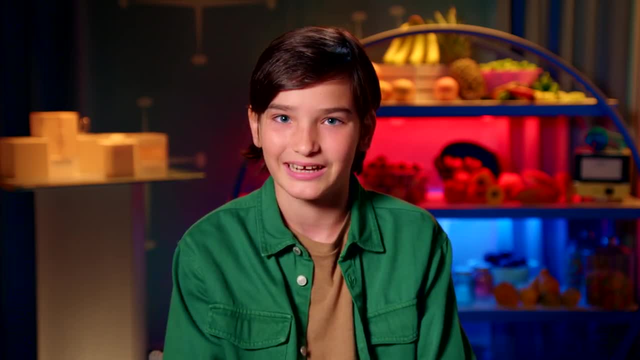 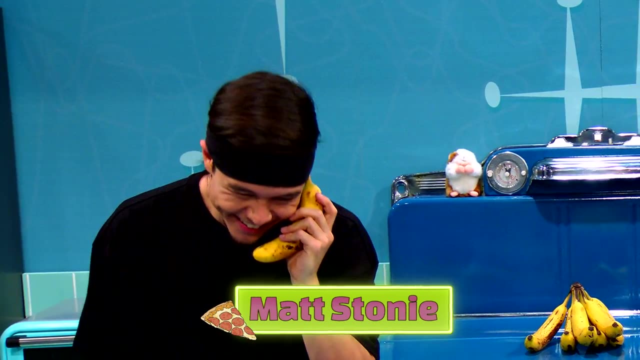 I was in awe of them. They were huge. I was not expecting it to be that tiny. Each teensy-weensy challenge will be judged by me, food vlogger Inga Lam and YouTube superstar Matt Stonie, who may be known for eating big, but here he's the king of tiny. 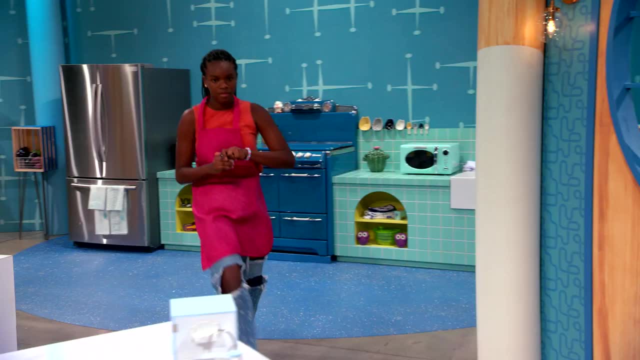 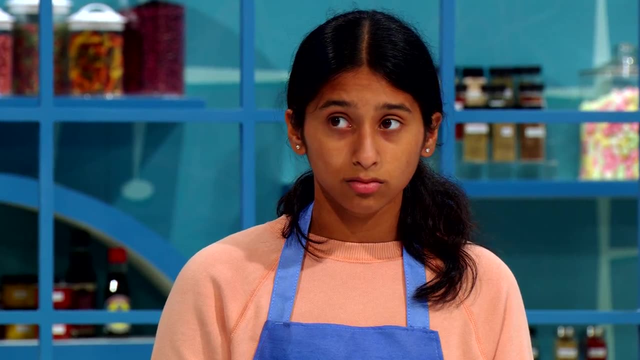 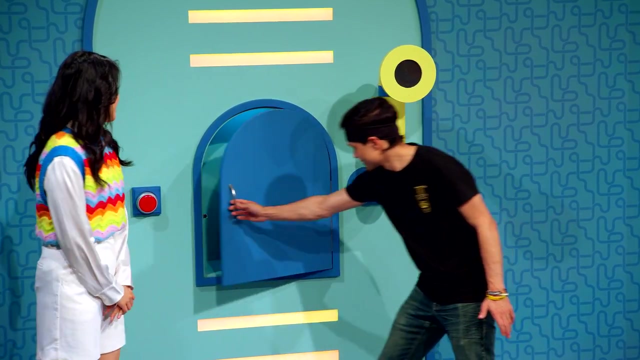 Today, our three young chefs head to the great outdoors in two challenges. Give me some more. and campfire classics. It's the biggest moment of their young lives and we will be crowning a winner. Oh, And stay tuned for some secret guests. 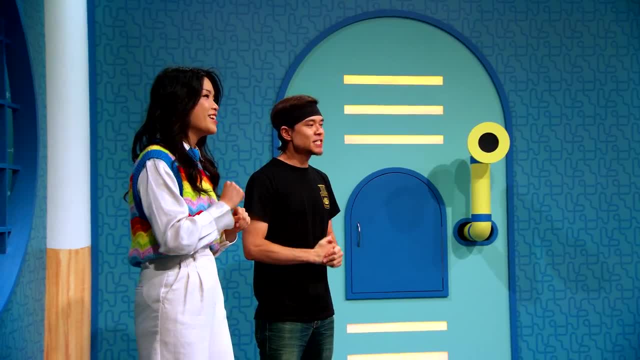 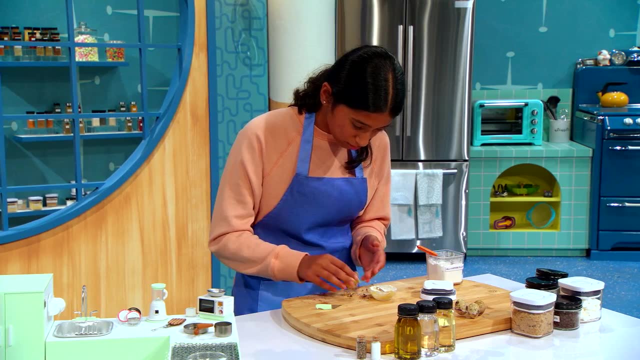 Here's a hint: They're furry and three inches tall. It's time to tidy. Our chefs are already hard at work. For the first challenge, we've asked the chefs for a new take on a campfire treat that goes back for 100 years. 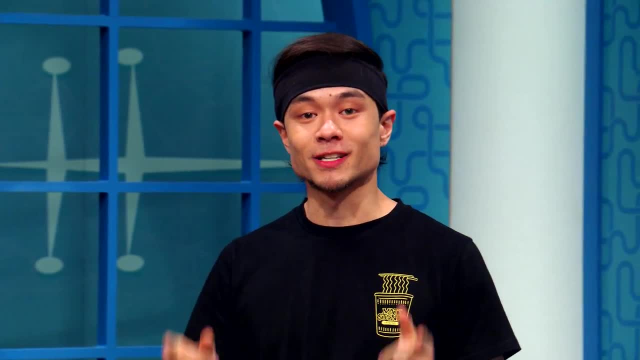 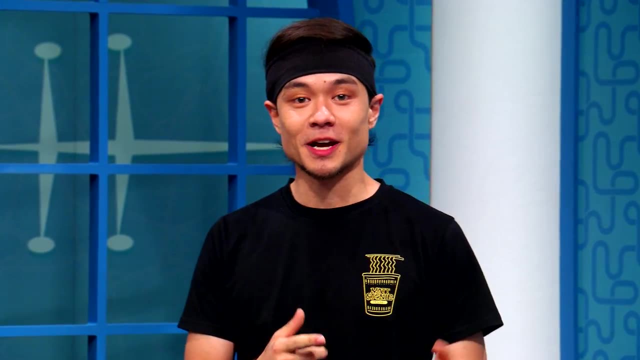 We're making s'mores today, baby, And the winner of this challenge gets an advantage in the final round. The chefs have 30 minutes to complete their s'more-inspired dish. Inga, let's get to know our chefs, Let's do it. 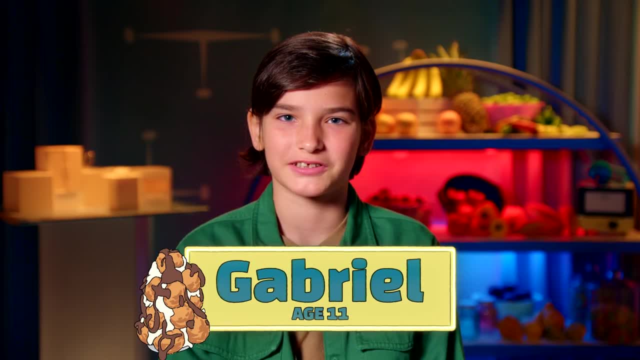 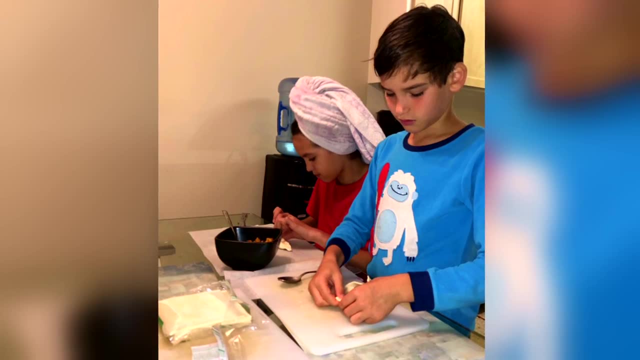 My name is Gabriel Gob. I'm 11 years old and I'm from Los Angeles, California, So I'm from Ukraine, and the city I'm from is Odessa. Everyone knows how to cook there. That's why I've been cooking from such a young age. 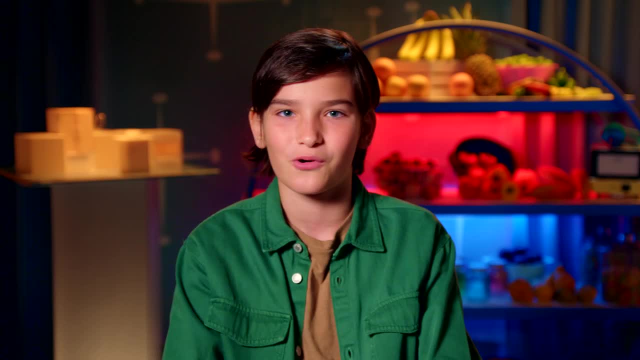 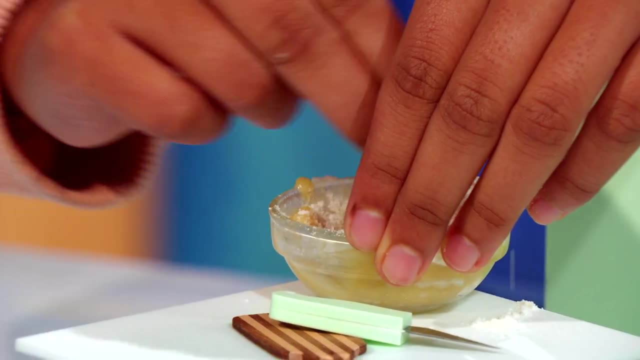 I was like three and I was helping my grandma in the kitchen making borscht or something like that. My name is Shreema Egela, I'm 13, and I'm from Owensboro, Kentucky. When I cook, I'm just in the zone. 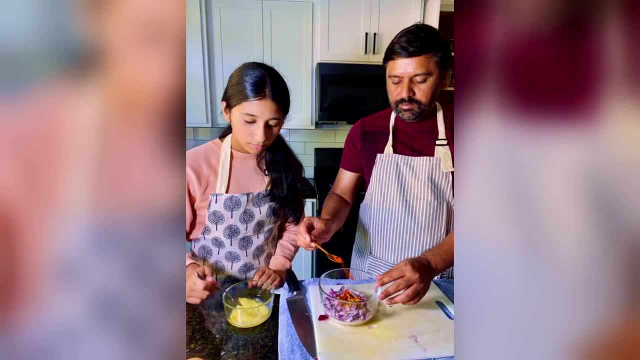 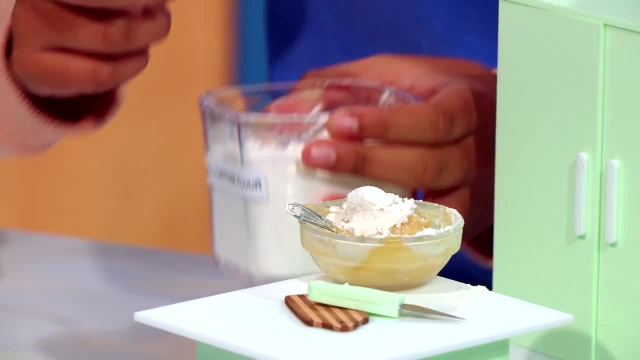 I forget everything else. It's my happy place. I don't have any other hobbies or obsessions, because this is my obsession. What I love about making tiny food is you get to see other people's reactions when you make this food. They're like: oh my gosh, it's so cute. 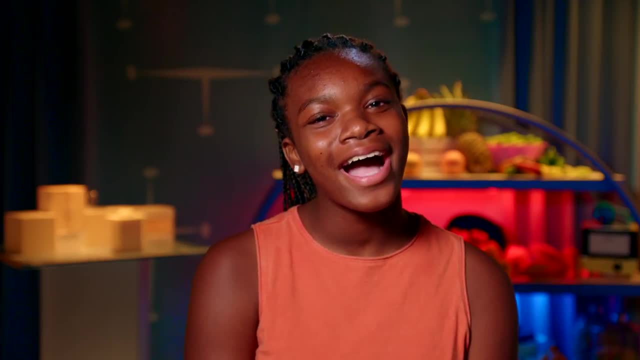 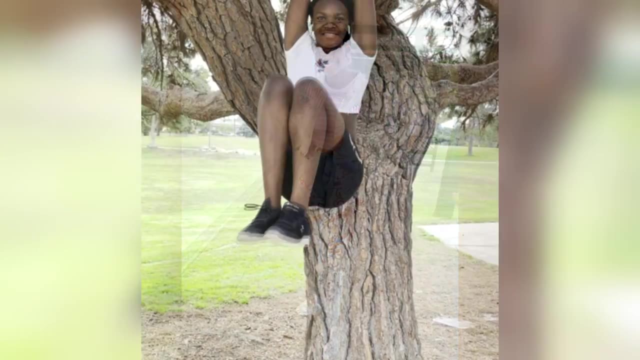 And I'll be like yup, I made that. Hi, my name is Madison Davis, I'm 13 years old and I live in Gardena, California. My family would describe me as fun, nice and sometimes energetic. I first started getting into cooking because my sister watches a lot of TV. 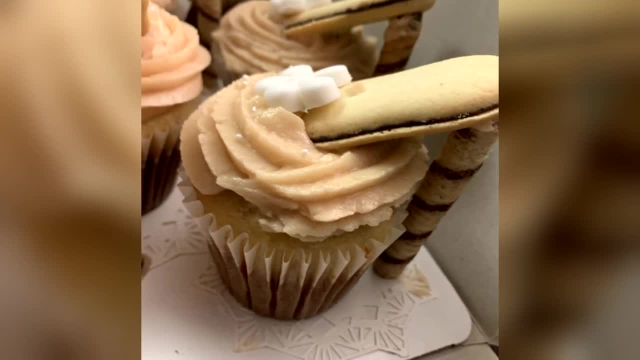 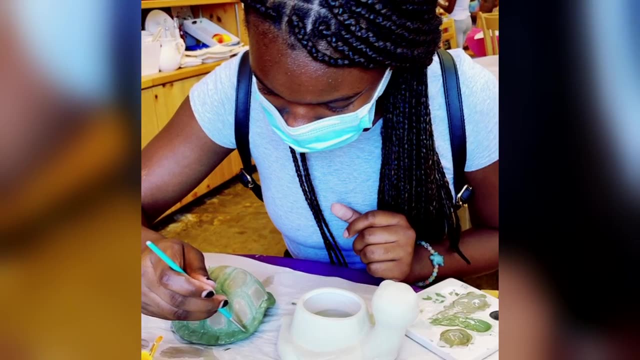 I watched a lot of cooking shows and I thought that was really cool. So then I started to make my own things. Then I decided maybe I'll try to do it tiny. I would say I'm kind of a creative person because I do really like drawing. 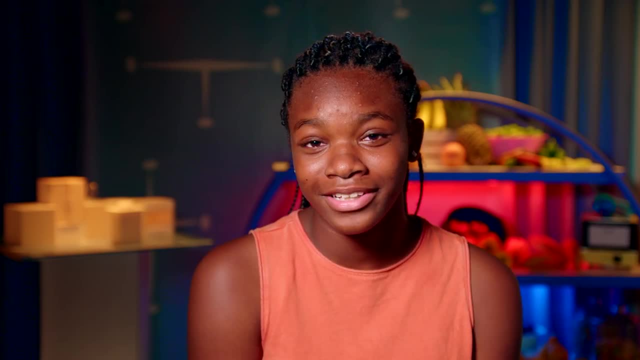 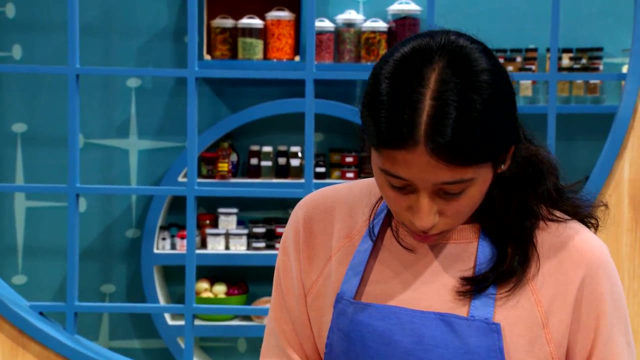 The best thing about making tiny foods is that you can be really creative. Stoney and I would judge their s'mores based on staying within scale, taste and how well they showcase each chef's personal style. So I'll be making a croquembouche, and that's a French dish. 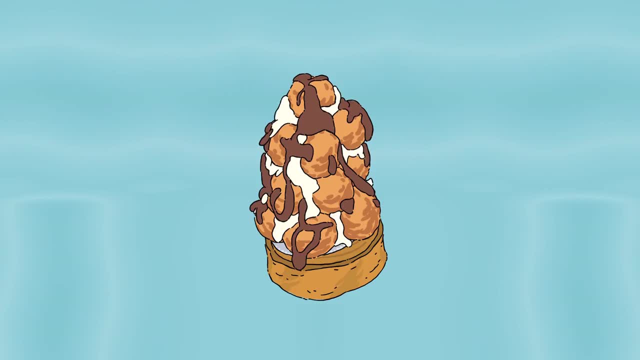 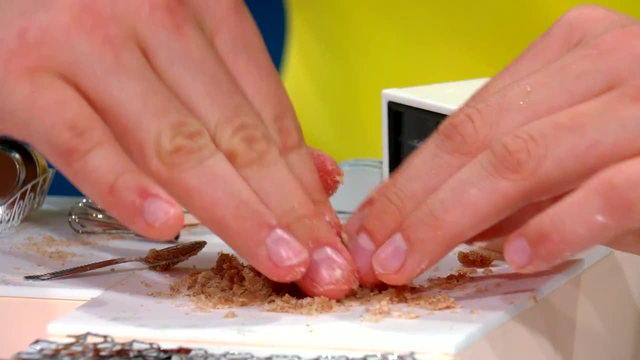 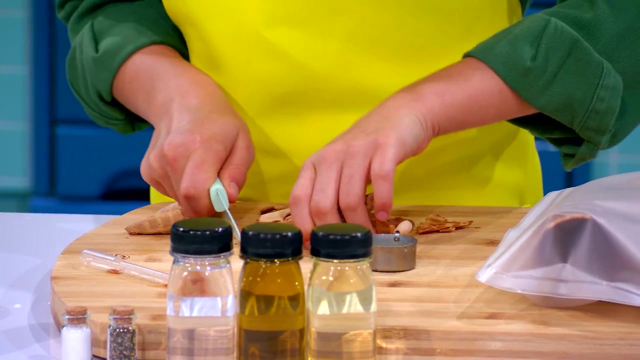 It is profiteroles Stuffed with custard And you would just take one out and then eat it. I think a real-sized croquembouche would be something like this, But since it's so tiny, I'll be making little graham cracker, little balls to stick onto the waffle cone with melted marshmallows. 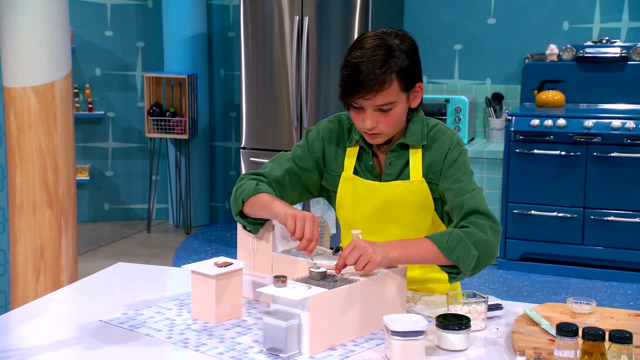 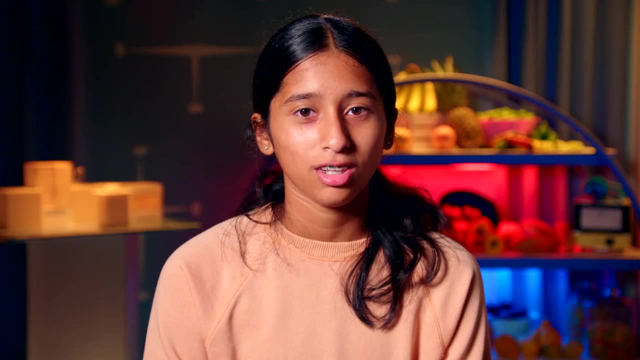 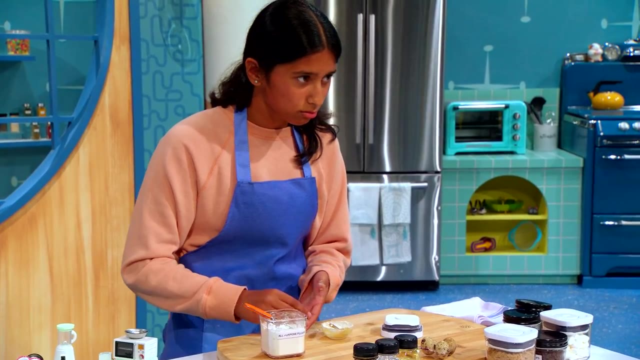 I'll be finishing it all off with chocolate. For this challenge, I'm making chocolate chip sandwich cookie s'mores with a peanut butter cup. I named it because that's what it was: Chocolate chip sandwich cookie s'mores. I'm really worried about my dough getting sticky because that's happened before. 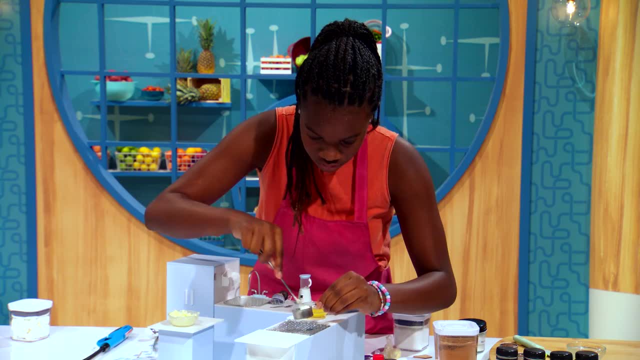 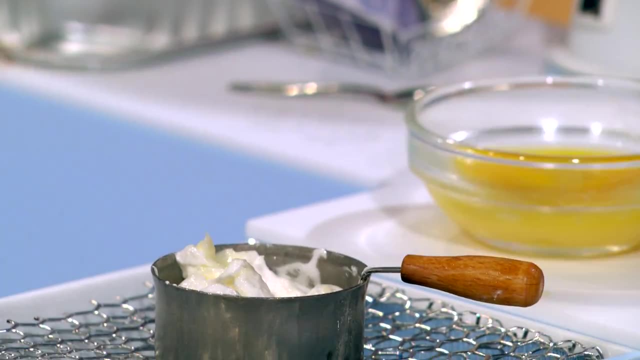 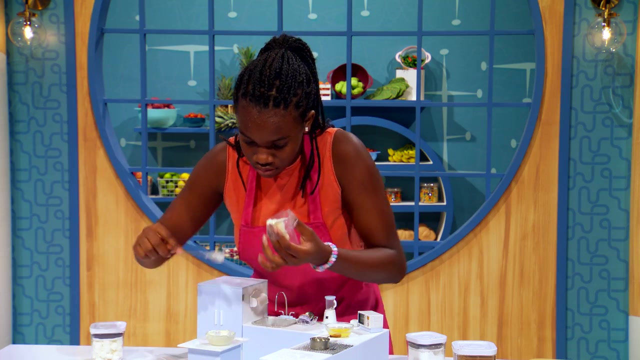 I don't want that to happen. For challenge one, I'm making a s'mores cake. I'm putting a vanilla cake, marshmallow frosting, then a chocolate cake, more marshmallow frosting and toasted marshmallows on top. When making tiny foods it's pretty hard to get the right measurements to make sure it has the right texture and everything. 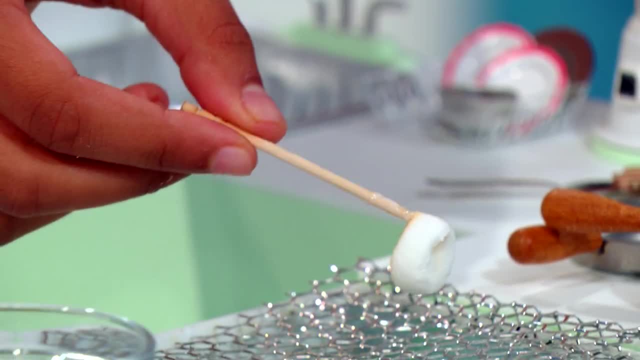 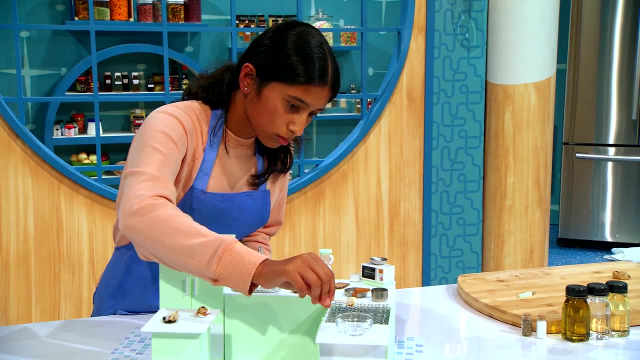 Five minutes left you guys. Only five minutes, Five minutes. My marshmallow kept on falling off the stick. I had to keep on getting new marshmallows, which was really annoying. So the dough for the graham cracker balls is burning. 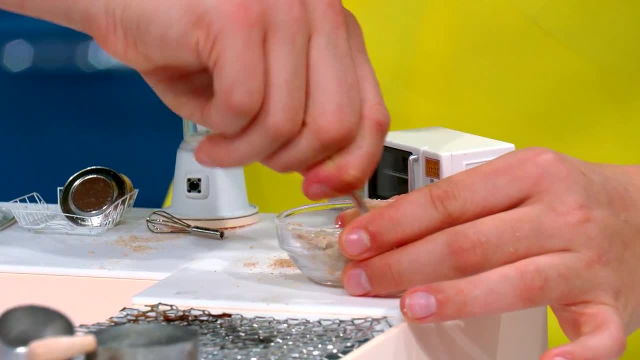 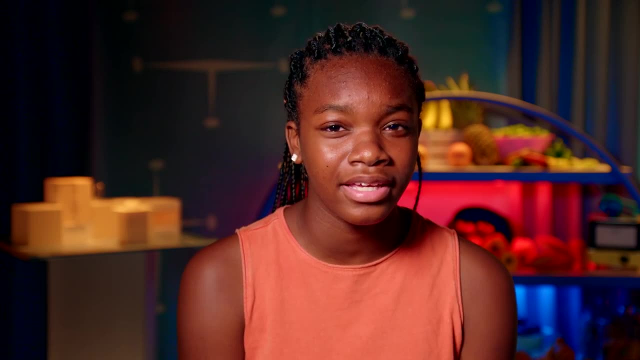 And I'm like, what should I do? And I'm like, okay, I'll make more dough, Hopefully that comes out well. I kept on thinking I need to make sure I oil the pan because the cakes wouldn't come out of the pan right and it would just not work out. 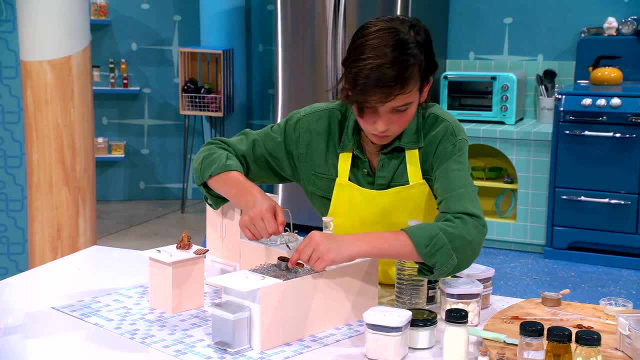 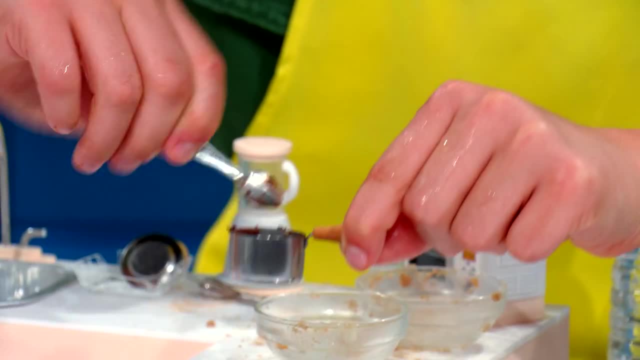 Oh, good For my croquembouche. I'm finishing it all off with chocolate, of course, because s'mores it's graham crackers, marshmallow and chocolate. All right, chefs, time is almost up. 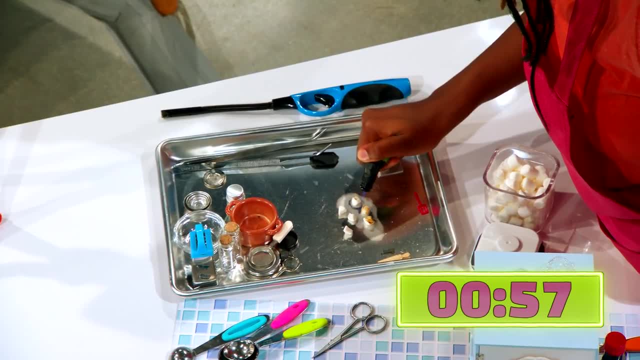 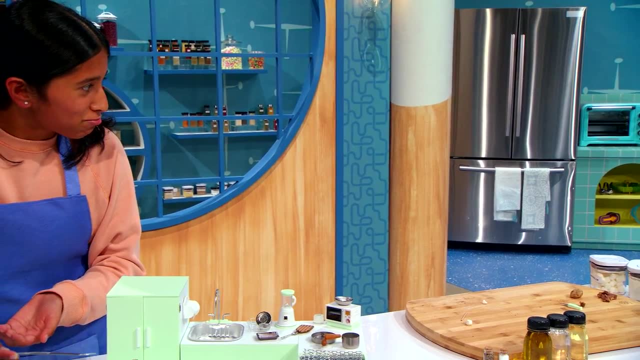 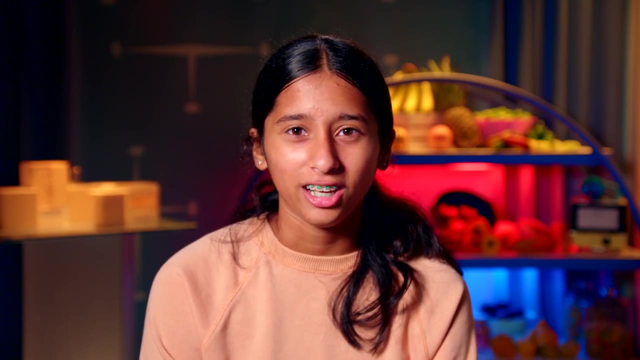 One minute left. I have to do this. toasted marshmallow. Oh, come on marshmallow, She just So. when I dropped stuff I was like, really Yeah, The hardest thing about tiny food is actually the size of it. 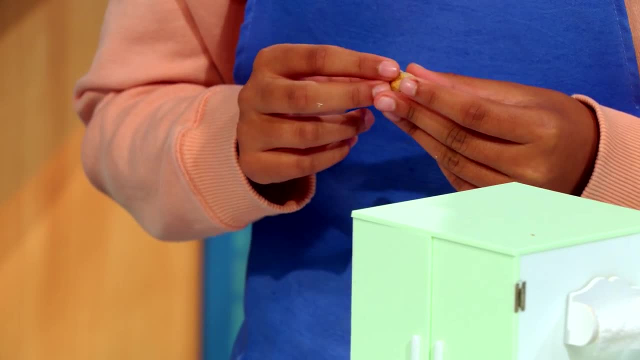 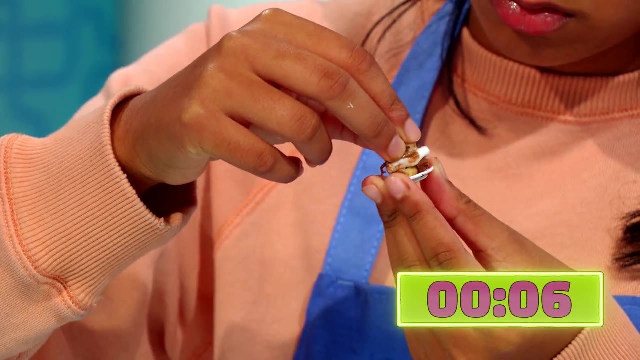 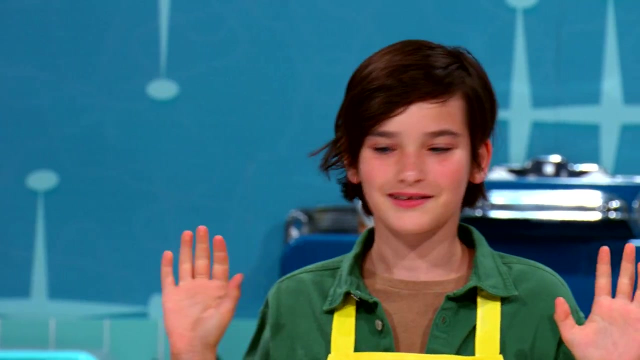 Everything is so small you keep on dropping it. You saw how many times I dropped that: Ten, Nine, Eight, Seven, Six, Five, Four, Three, Two, One And zero. Put down your cooking tools. tiny chefs. 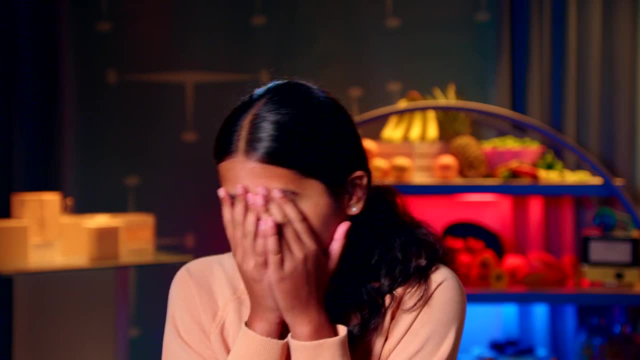 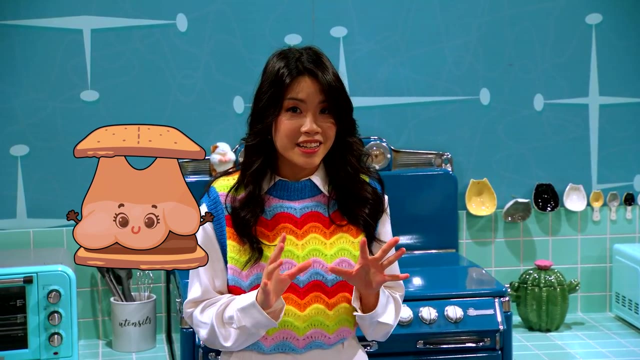 Oh God, what a mess. I still have to look. No, I can't look. Here's a tip for you. The key to making the perfect s'more is to cook the marshmallow fast on high heat, so it's crispy on the outside and then soft and gooey on the inside. 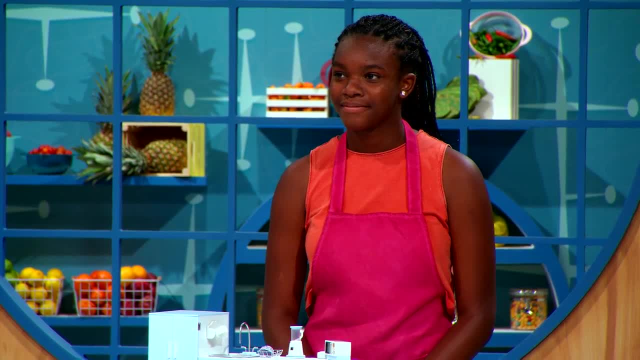 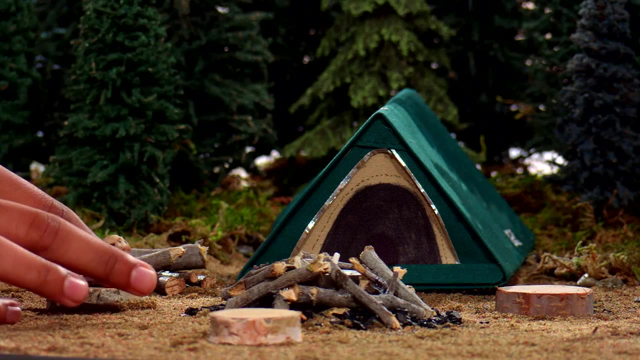 All right, chefs, I think it is safe to say that your skills today have impressed the heck out of all of us here. Srimaya, come show us your delicious tiny food. Tell us what we have here. So I made cookies, and then I put a chocolate peanut butter cup on it, and then I cut down a mini one. 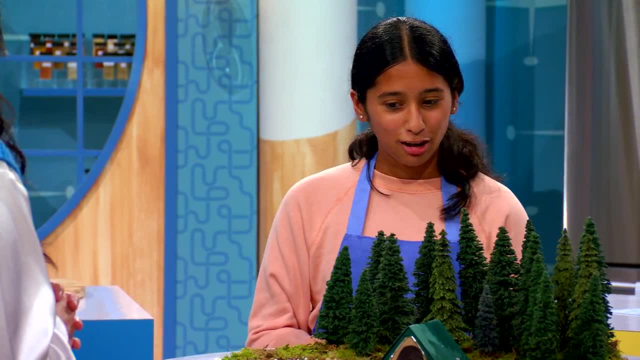 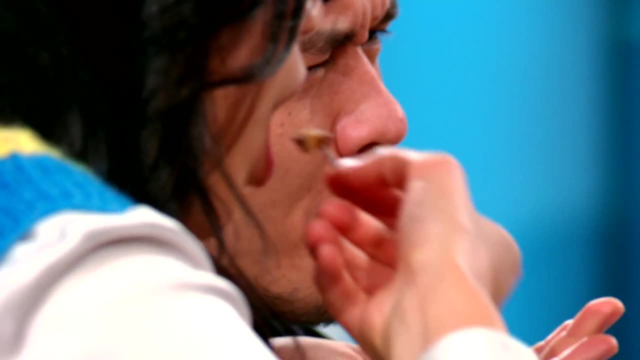 I cut down a mini marshmallow, as it wasn't small enough. I can eat cookies in my sleep, so I put those on top. Yeah, let's dig in Cheers, Mmm, Peanut butter and chocolate Right away. it's the peanut that comes through. 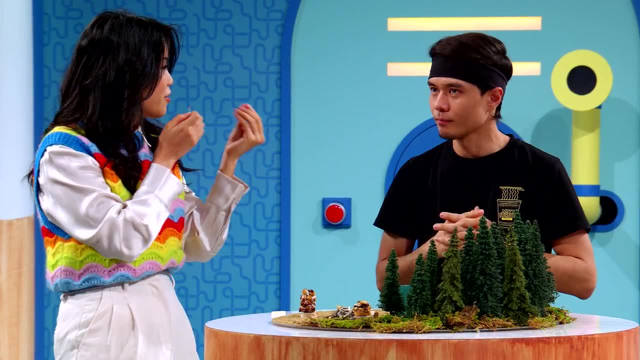 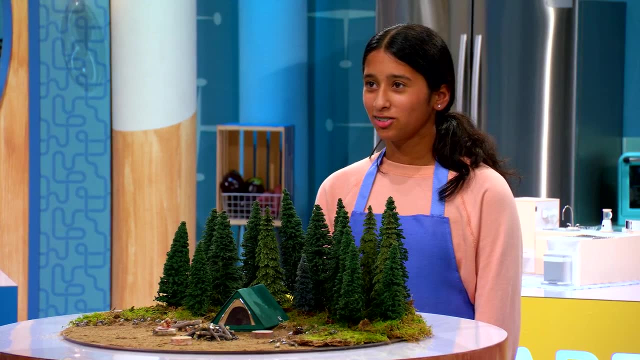 The texture of it: not too doughy. It kind of has a bit of a chew to it. that goes really well with the marshmallow. The cookie was cooked perfectly. It crumbled just as you'd want it to Do. you feel like you're eating a s'more, but cookie version. 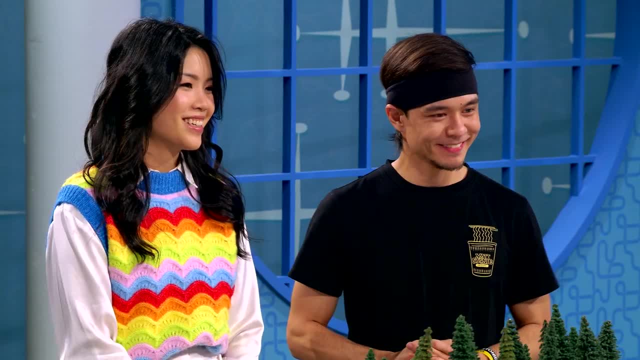 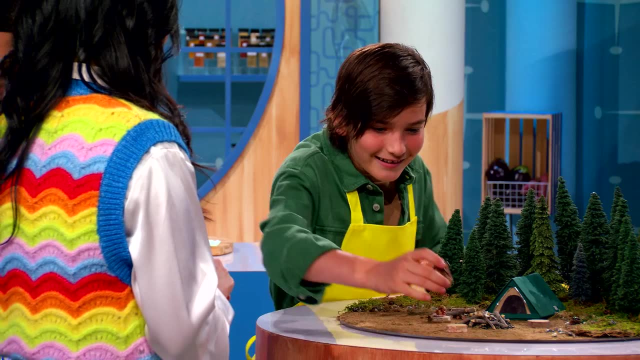 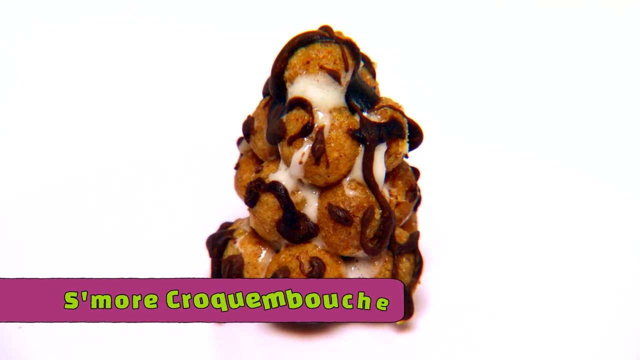 100% Right. Thank you, Thank you. Thank you, Gabriel. you ready? Look at the little tower of cookies. Holy moly, What is that? What you see here is a croquembouche, only s'more croquembouche. 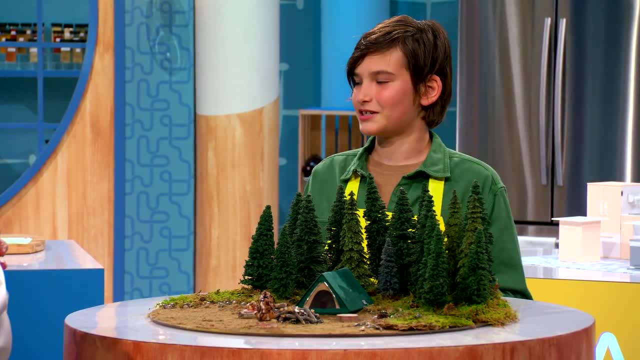 Croquembouche, Croquembouche, croquembouche. What is a croquembouche? A croquembouche is like a tower of puff pastry. Yes, And it has this cream, which actually the cone itself is filled with the cream. 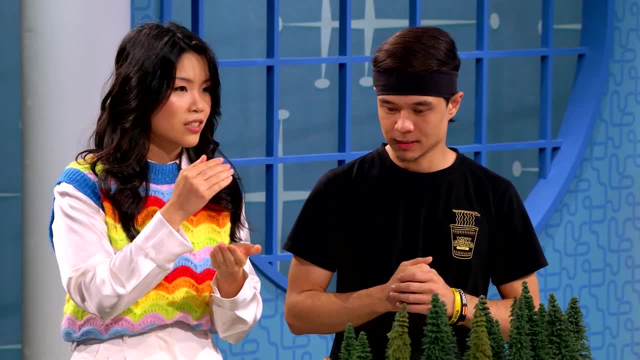 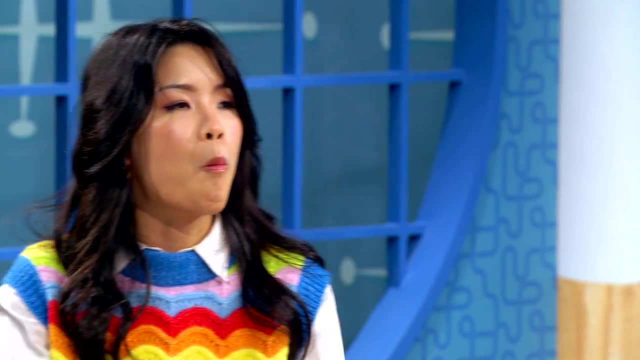 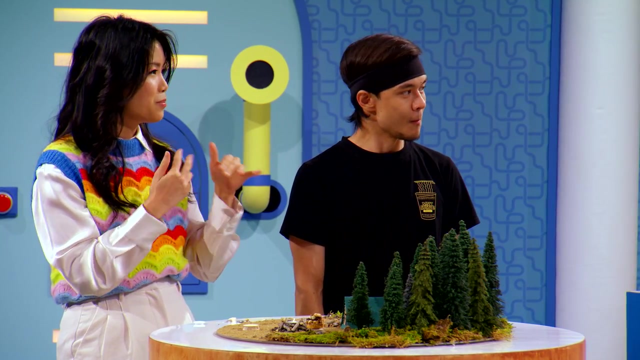 Then you have the cookies and then you have the drizzle. Yeah, Okay. Well, here you go. Chocolate marshmallow. I'm getting so much of the cone Right. The cookies. I like that you pivoted and made it into like a more like graham cracker texture. 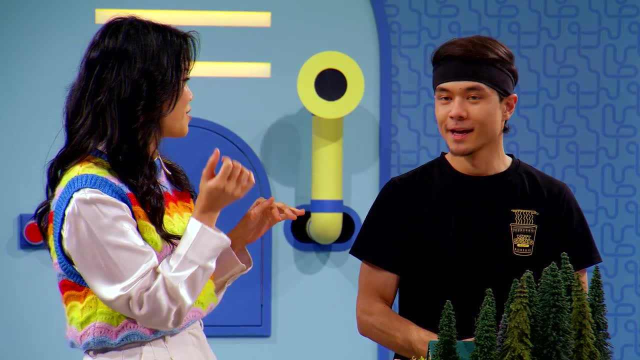 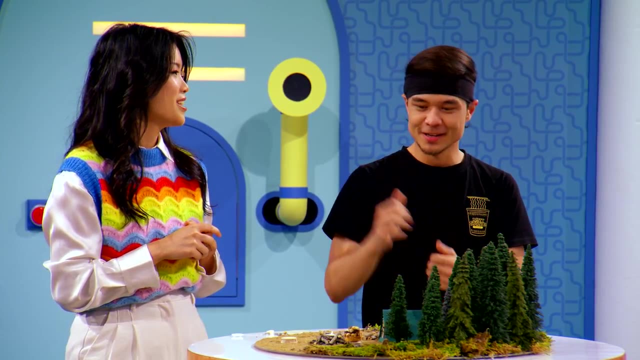 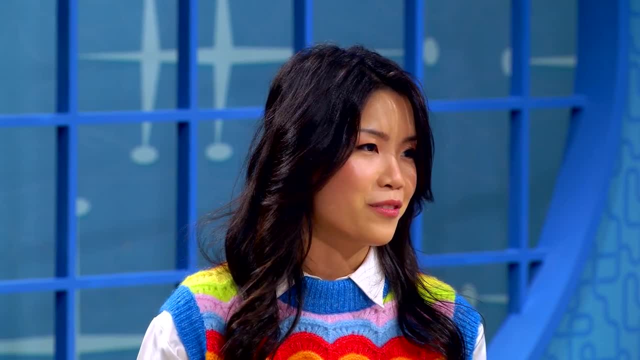 It's nice, It's nice. Oh, Gabriel, I just want to say you should be very proud of yourself, Very proud For being able to pull that off in such a short time. Thank you, Gabriel, so much, Thank you. 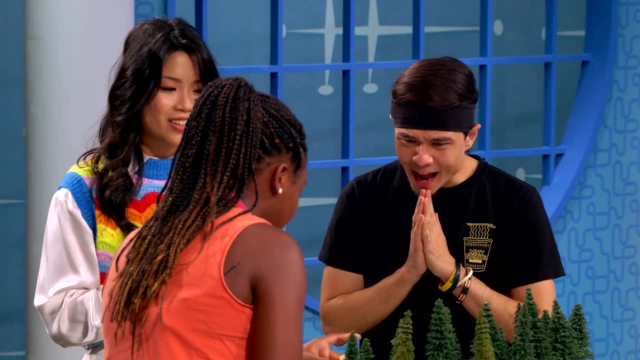 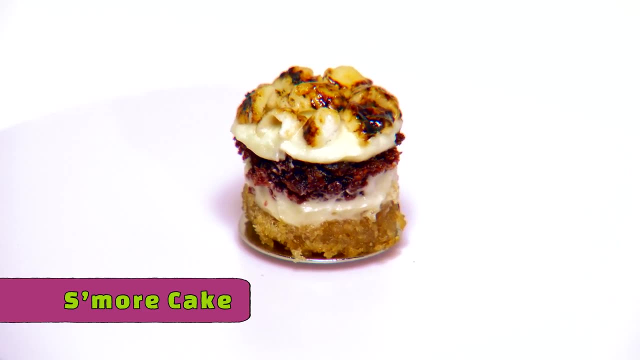 Thank you All. right, Madison, Here it comes. Oh my Wow, Look at this. Wow, Please describe this to us. It's vanilla cake, on the bottom marshmallow buttercream, then a chocolate cake, more buttercream. 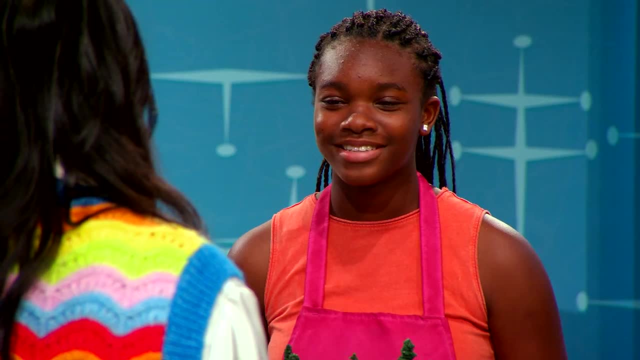 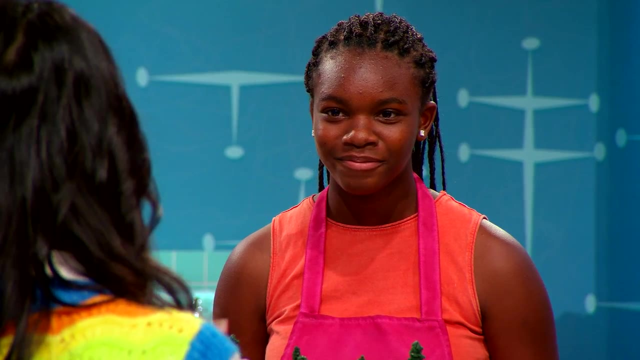 and then I cut up the marshmallows and then I blow, torched it, Because that's like my favorite part of s'mores is the roasted marshmallow. I love that. You really like kind of channeled the camping spirit. I've never had a cake to myself. I just want to say 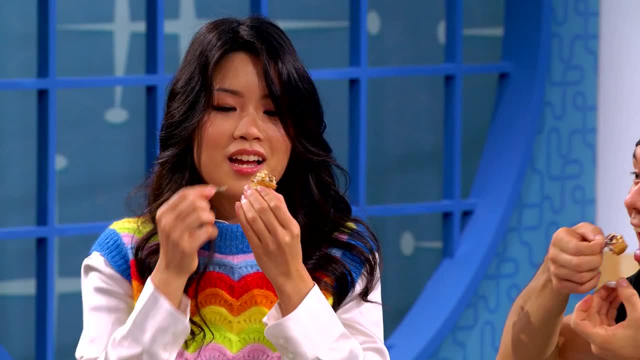 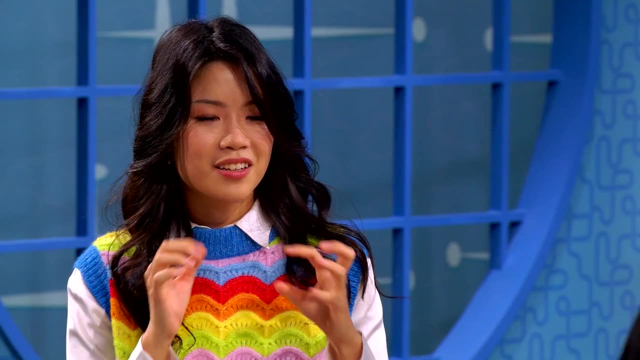 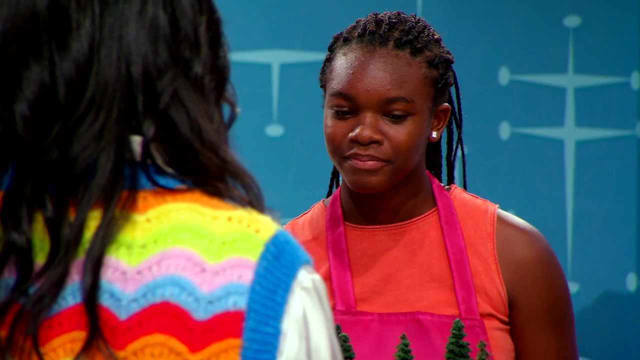 I have, Of course you have. Okay, Are you being transported to like camping right now? That roasted marshmallow flavor that you were talking about really comes out Perfect golden marshmallow that you cook on the campfire, One that you're proud of. 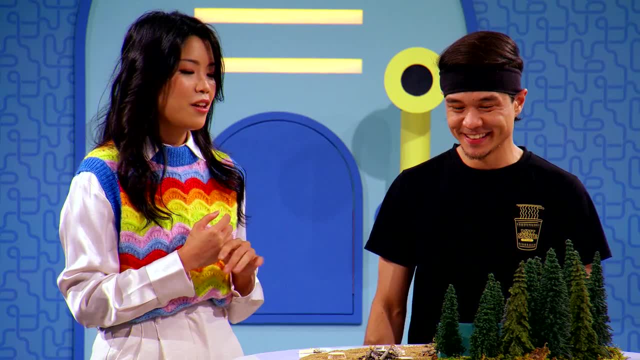 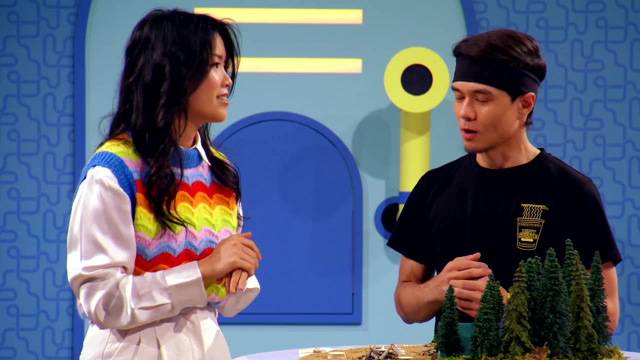 And then the cake, kind of fluffy. You get that too. The only thing I will say is, though, I could not taste the difference between the vanilla and the chocolate, but it's very, very good bite. Oh, very good bite. 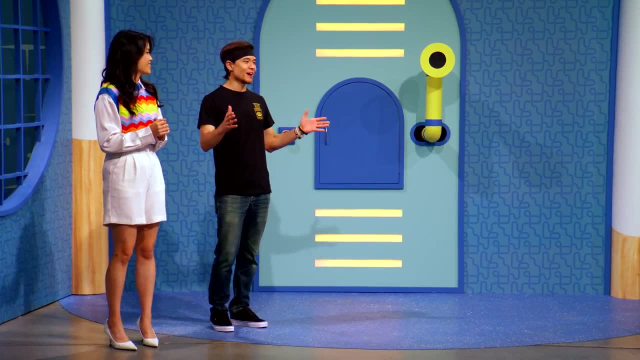 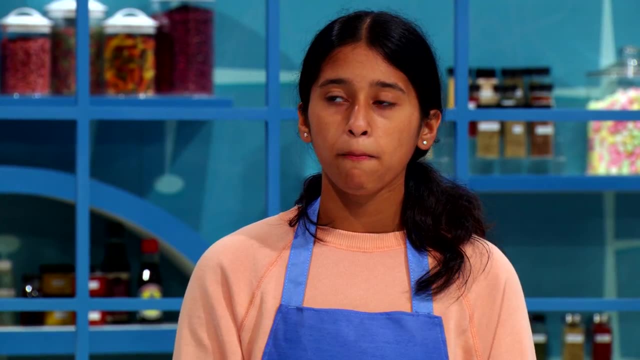 Okay, Thank you. Thank you. All right, Chefs, your skills today have impressed the heck out of all of us. I mean, all three of your dishes were fantastic and delicious, but we had to choose the big winner of today's tiny challenge. 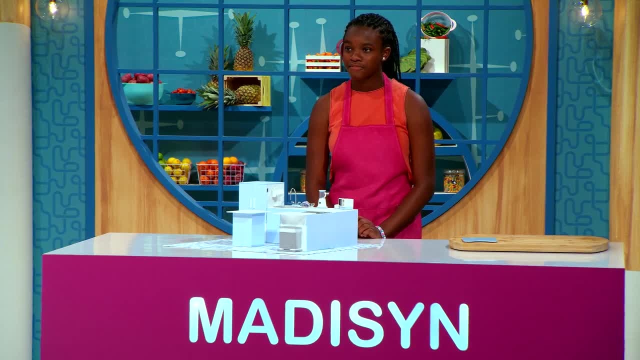 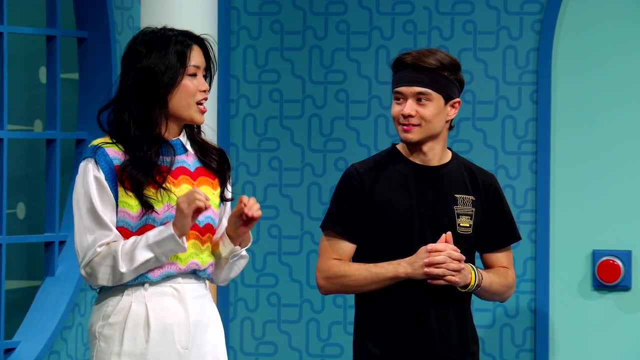 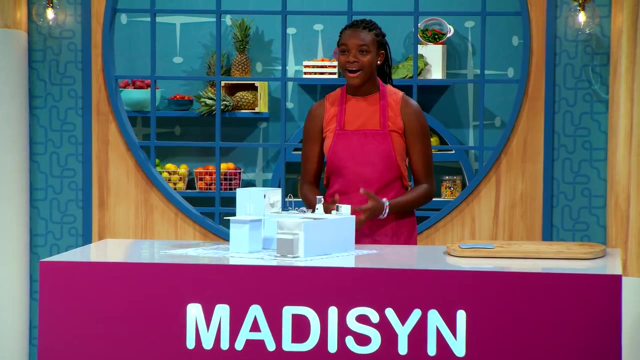 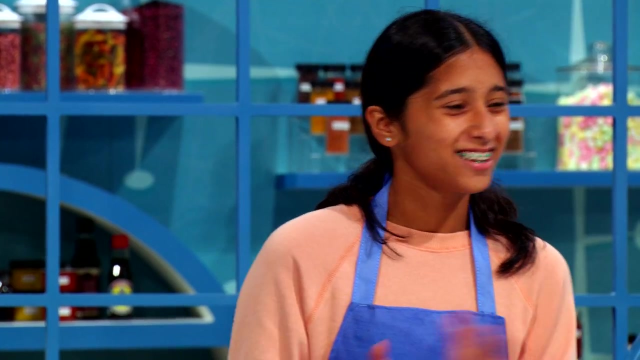 For being able to downsize their dessert perfectly, give us incredible taste and showcase a little bit of their personality. Our winner for this first challenge is Madison, with her incredible s'more cake. Congratulations, Great job. And now it's time for my favorite part of the show. 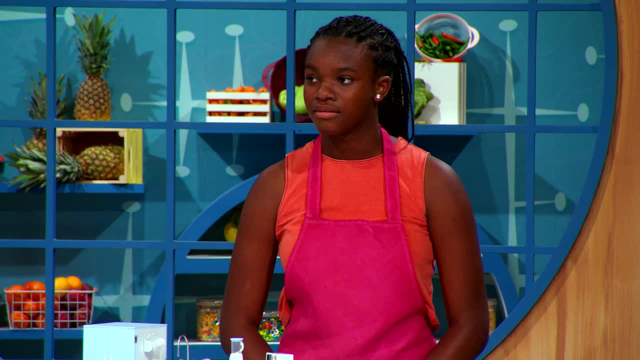 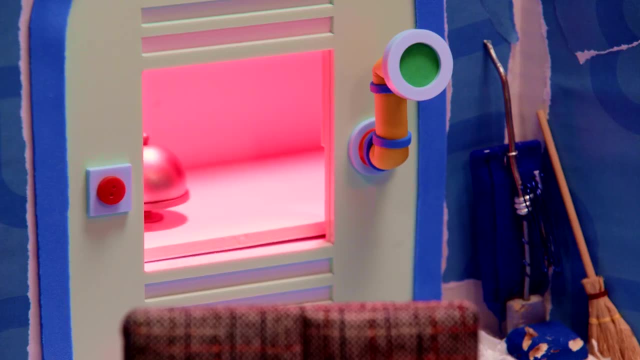 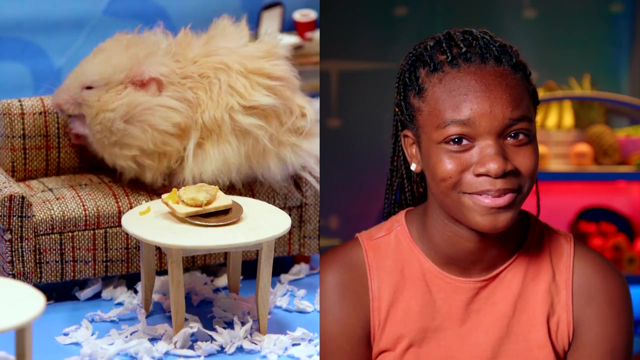 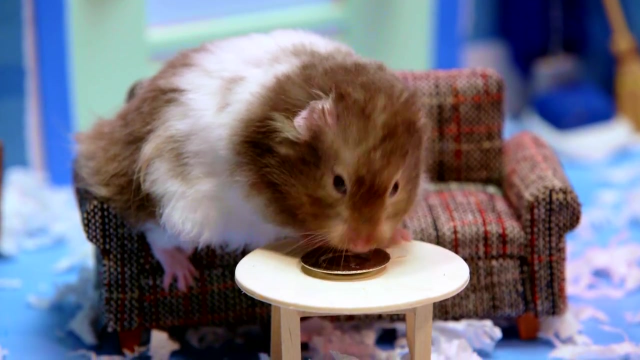 Let's give a taste to our special guests who will be helping us in the final challenge. I would say I'm a pretty big hamster lover, so the opportunity to cook for them is like wow, Maybe one of the hamster judges can come home with me and be my pet. 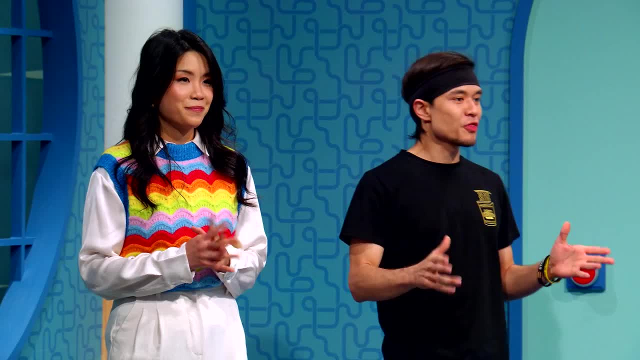 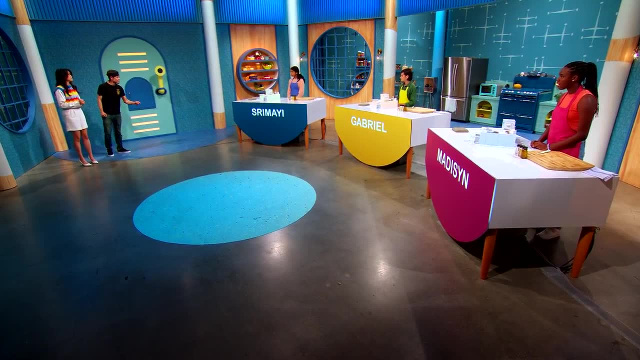 Dad, can I keep one? And now things are about to really heat up as in fire, because that is what you are going to need to cook this next meal. Are you guys ready for cooking? Are you guys ready for campfire? classics: 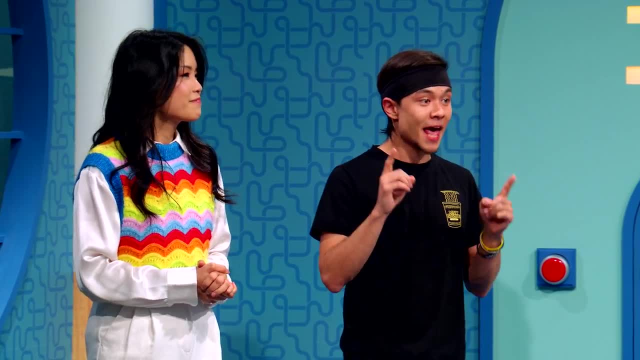 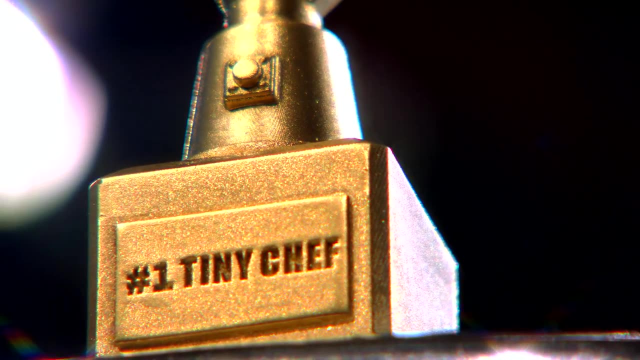 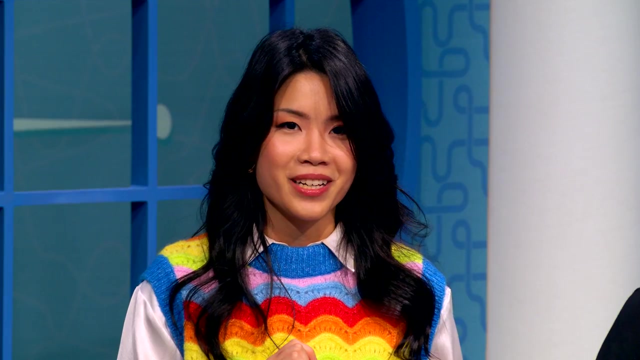 Yes, we are. This challenge is for all the marvelous and that beautiful number one: tiny chef, golden blender, trophy Chefs, your goal is to make a full campfire classic meal. but there's a twist, Stoney. why do you look so shocked? 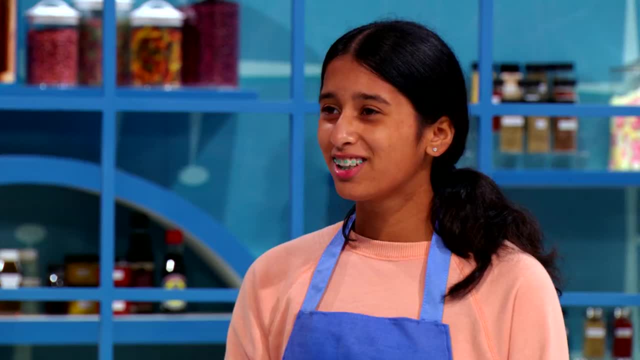 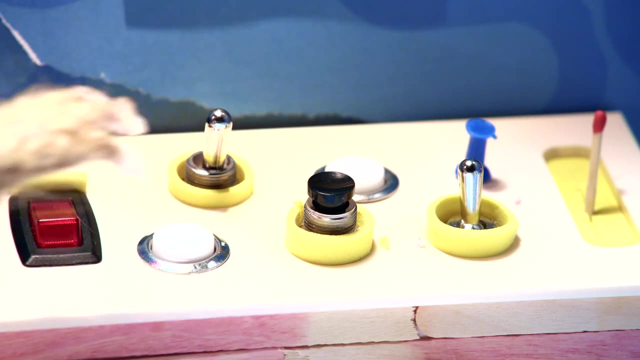 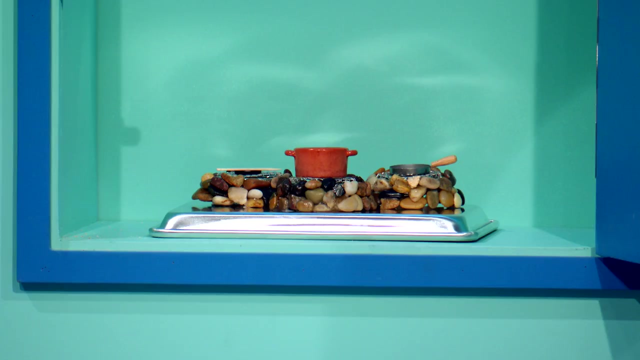 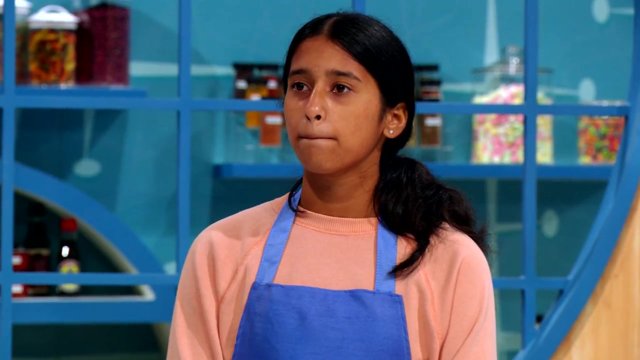 This is our show. I was a little late to the production meeting this morning. My bad For this challenge. you will not be using the stove in front of you. Our hamster friends have three campfire tools: a griddle, a grill and a Dutch oven. 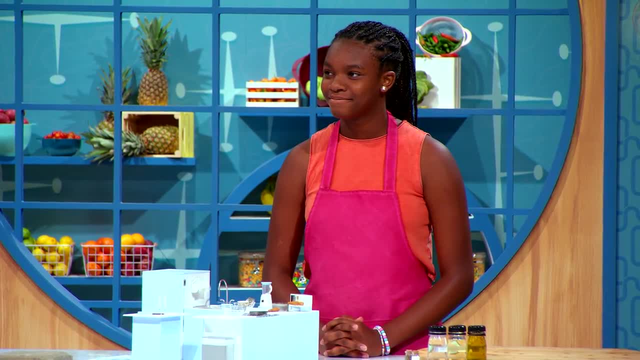 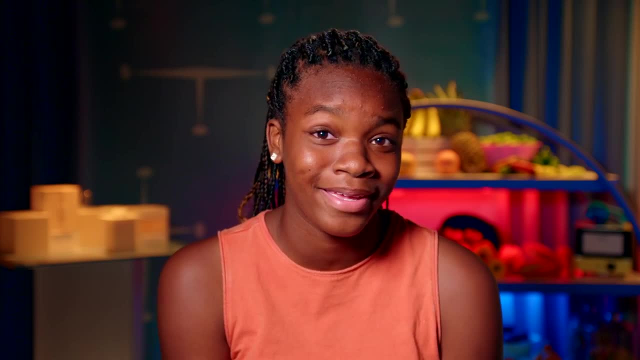 So, since Madison you won, you get to assign the tools. Going into the second challenge, I'm excited that I won. I'm excited that I won the first one, but I'm a little nervous because I'm not as good at cooking as I am baking. 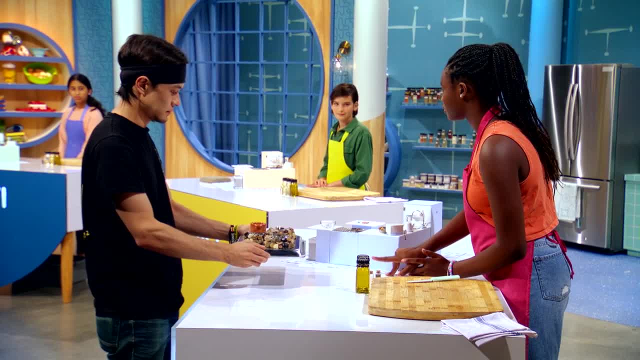 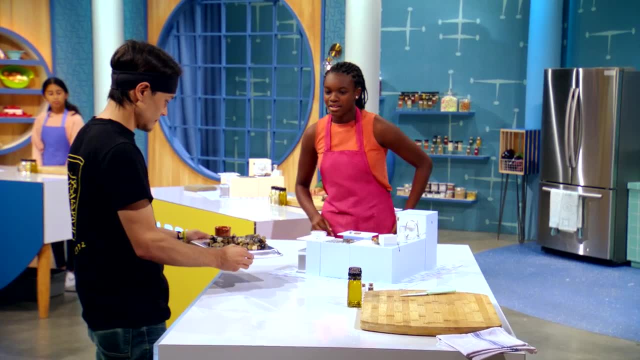 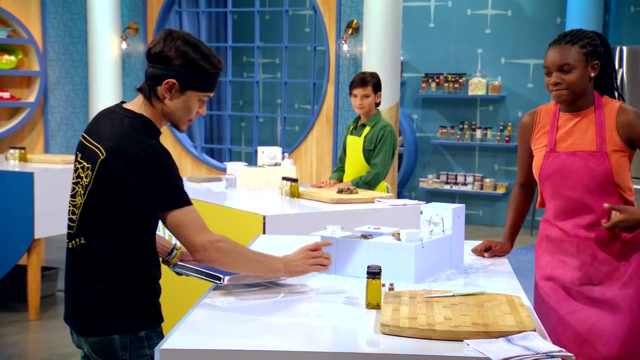 I'm going to give the griddle to Gabriel, because I know he likes cooking more than baking. Now, this is my natural habitat, And then I'll give Shamari the skillet Skillet, All right, And then you, Madison, get the Dutch oven. 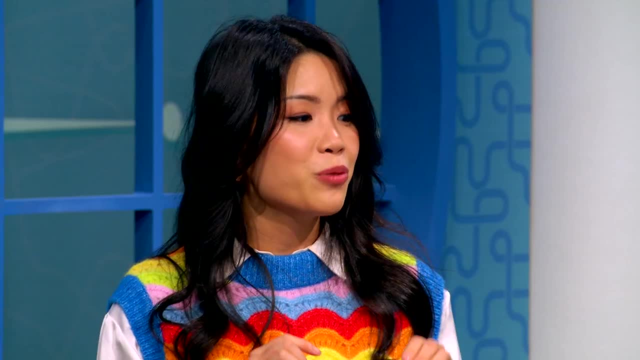 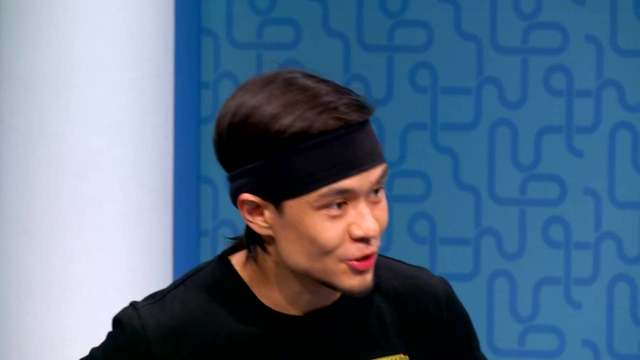 Yes, In this challenge, you will be judged based on your technique and your skills. Your technique, innovation and, of course, flavor. So you've got your tools. It is now time to cross the finish line. Ready, set go. 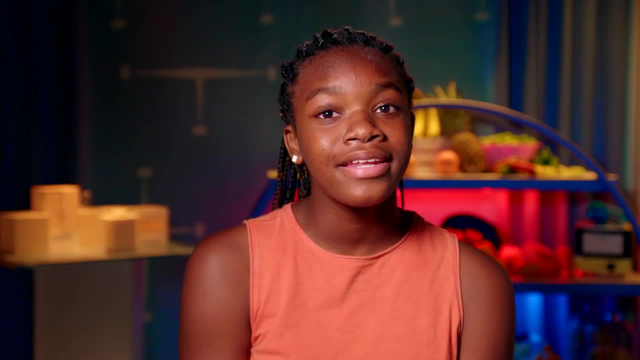 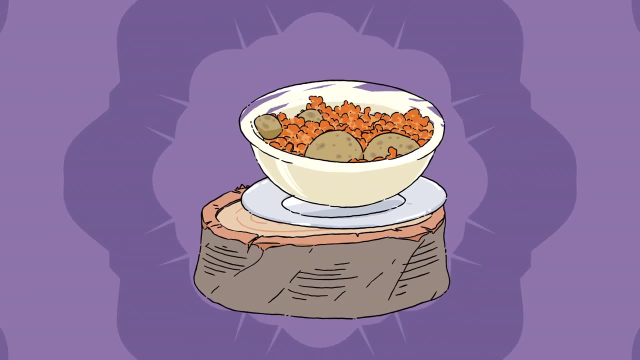 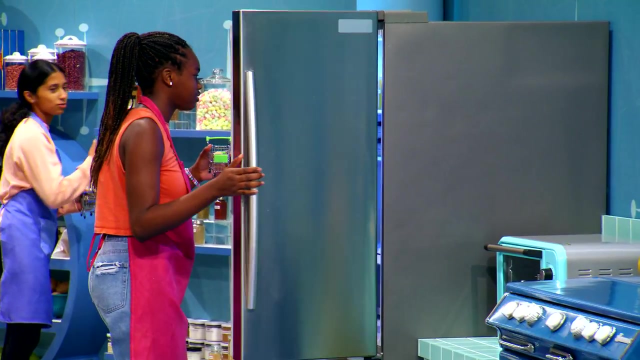 You only have 60 minutes to create your dish. I decided to use the Dutch oven because I was planning to make a corn stew And I feel like that's easier to make in a pot With sweet corn, heavy cream, lime, the potatoes, goita cheese, cilantro and- the secret ingredient- cheese. 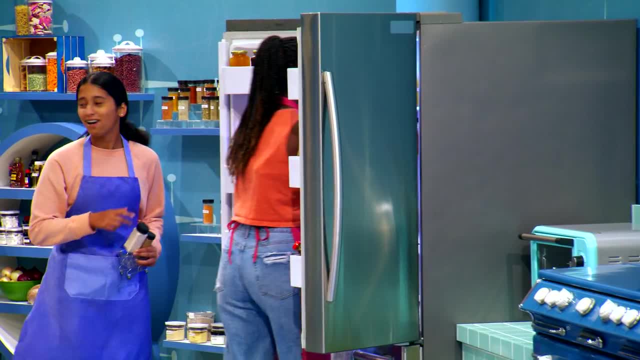 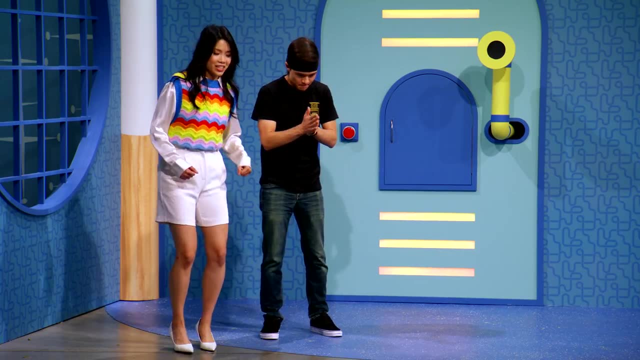 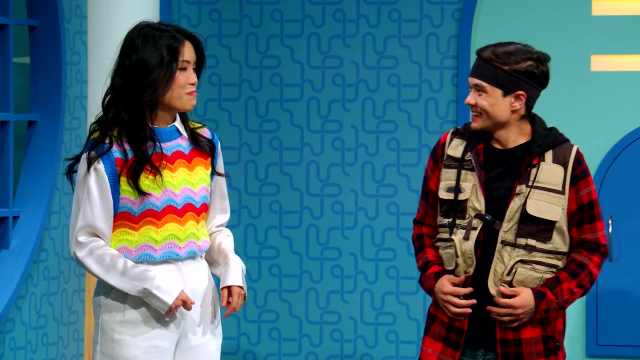 Did you taste the chili powder? I'm trying to make sure I get different kinds of flavors that go together, So I'm hoping that puts me up at the top. All right, At the tin there's nothing more appropriate. It does look very camping style. 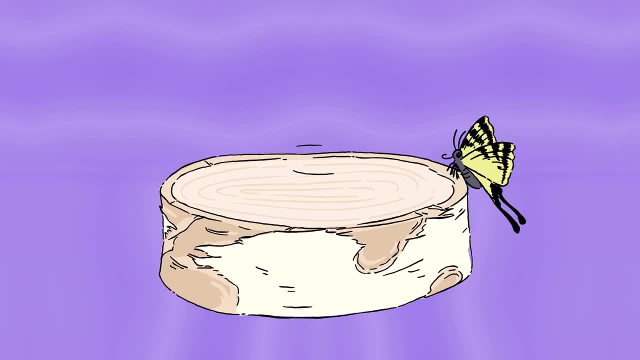 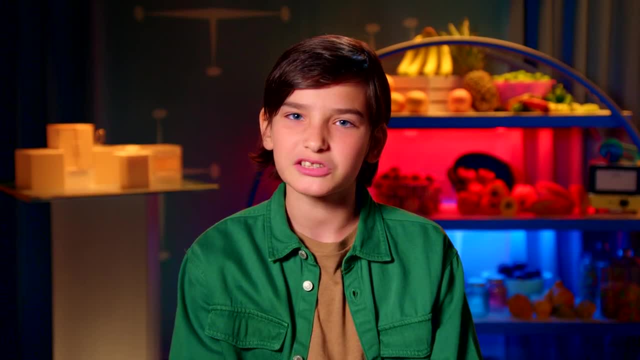 So I'm going to be making a marinated salmon in beetroot, which will give it a nice pink color. All right, I went to Alaska this one time, And me and my dad- there was so many salmon. We were just catching one after another. 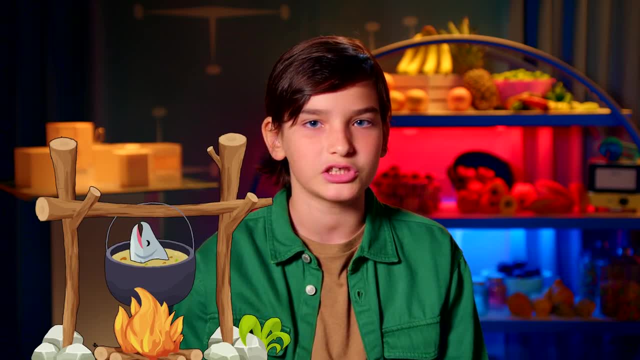 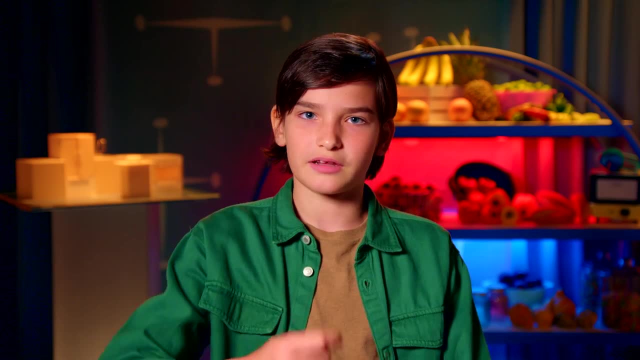 And after that we went camping and we made this amazing salmon dish. So that's how I got the inspiration. I'm also thinking of adding a pickled beetroot and then curl it up into making like a tulip or a rose-looking figure. 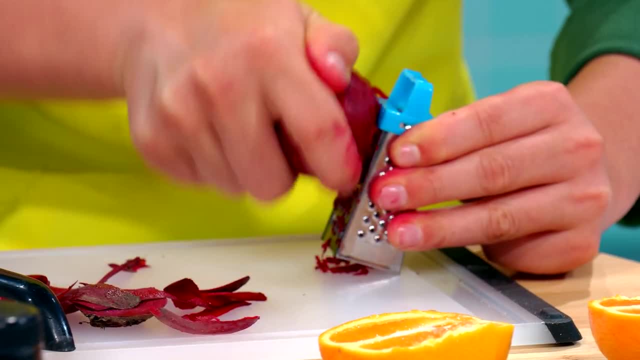 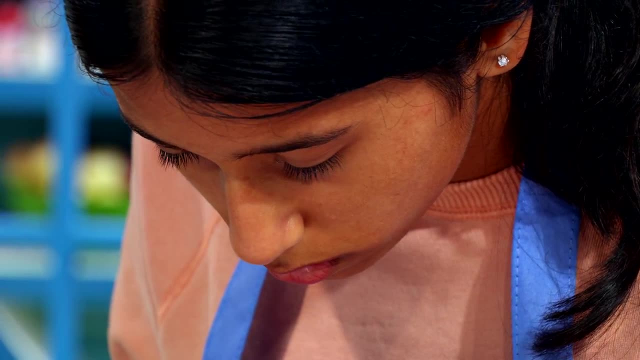 My traditional dish in my country is something called borscht or red beet soup, So me and my grandma would cook that. so much So, of course, I would have always been using beet. For the second challenge, I'm much more relaxed. 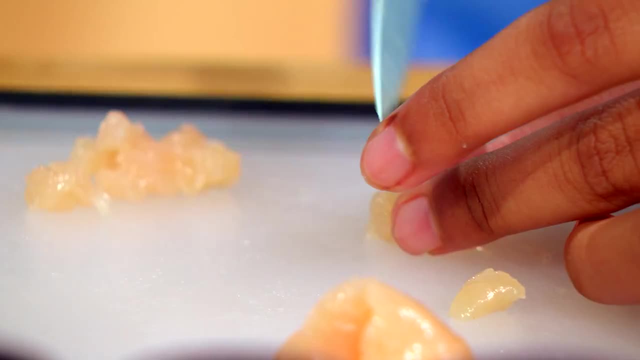 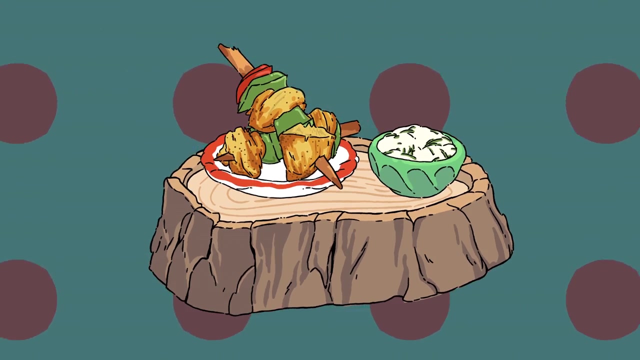 And I've gotten to know where everything is. So I feel like I'm going to do much better. I'm making chicken skewers with red onions, green bell pepper and a dip. For my dip I have sour cream, mayo, garlic powder. 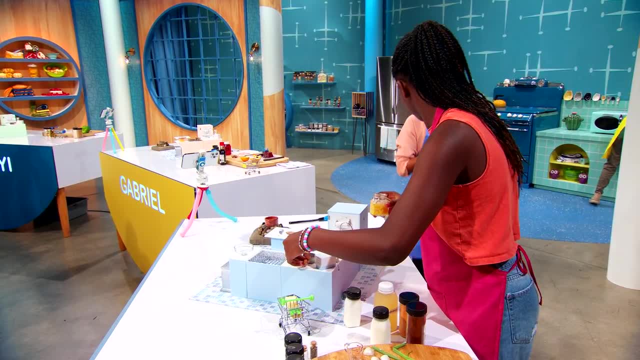 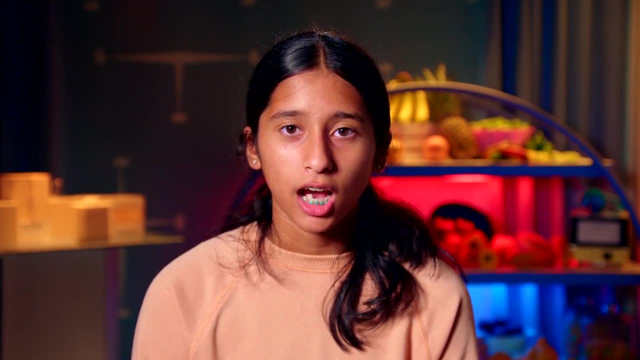 And then I'm going to sprinkle some dill weed on top to make it look pretty. Madison, I need your chili powder Here. bring it back. I'm very confident this round because I know what I'm doing And I don't have to measure out all these ingredients. 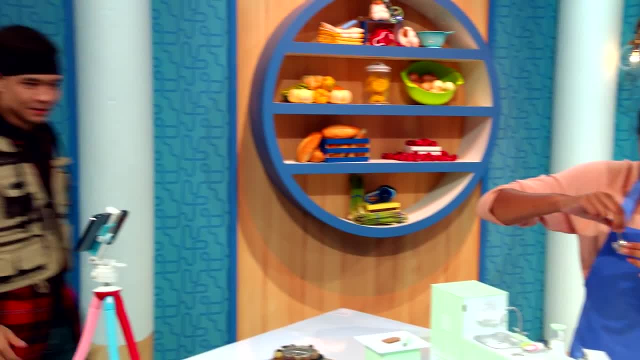 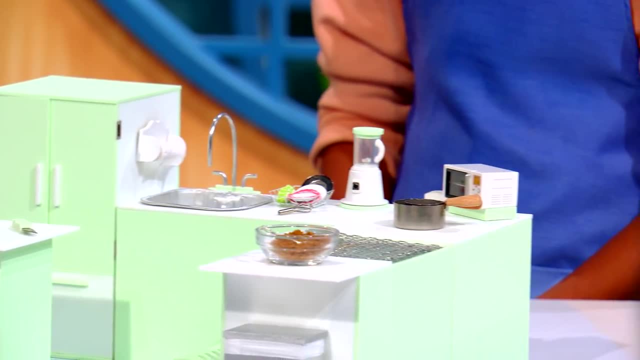 So I can just eyeball it, even though I'm not the best at that. Shree. what's going on? It's going great. What is this seasoning over here? So I have garam masala, salt pepper and chili powder. 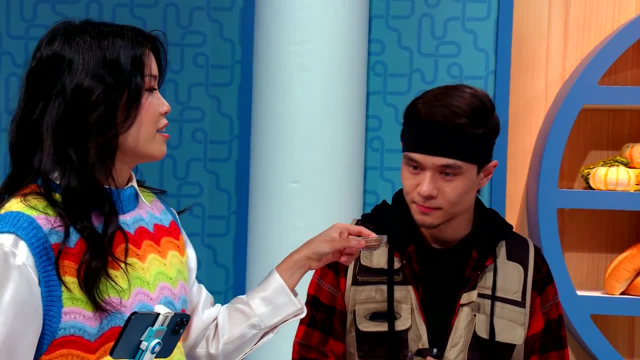 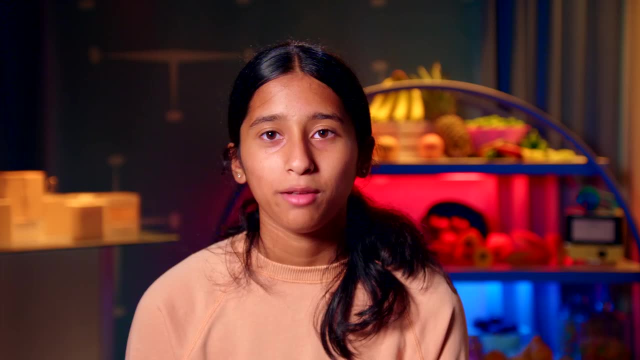 OK, can I smell it? Yeah, go ahead. Oh man, you got to. Oh man, I think the judges are going to really be blown away by the spices that they're going to feel in their mouth. Tell me more. 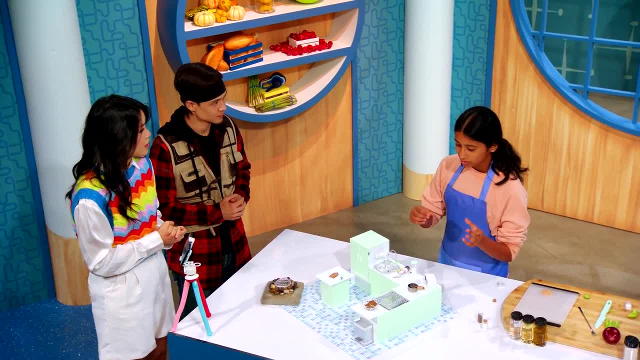 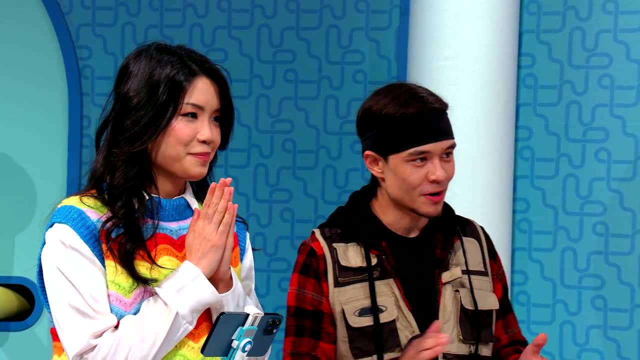 Is it your dad's recipe? When we grill, we put some of the garam masala on top. I don't know what else he puts, because it's a secret recipe. Oh OK, A little bit of a tough question here. 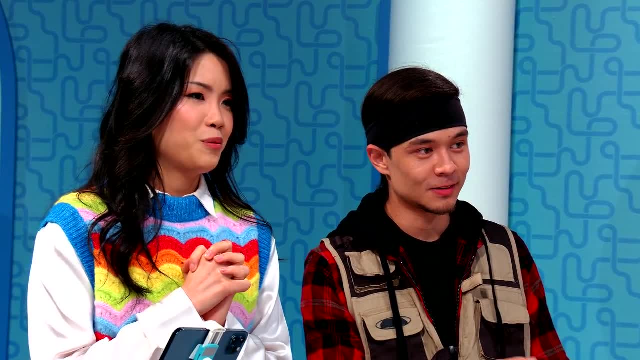 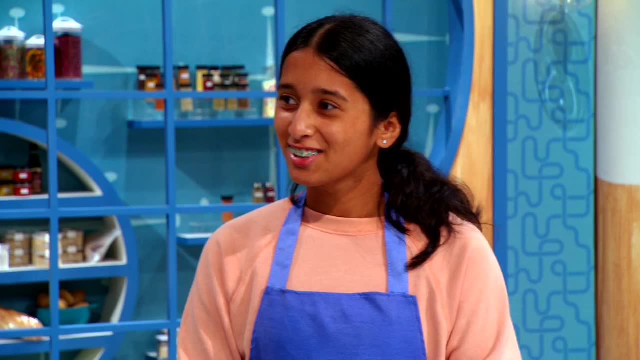 Who would you say is the better chef, yourself or your dad? Me? Well, he makes traditional food, OK, But I bake and stuff. I'm all about confidence. New school versus old school. That just left your ass, Thank you. 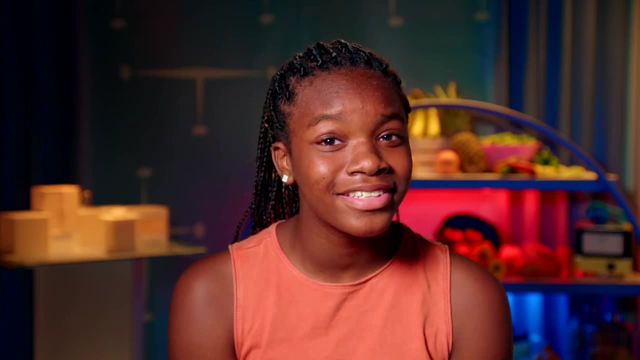 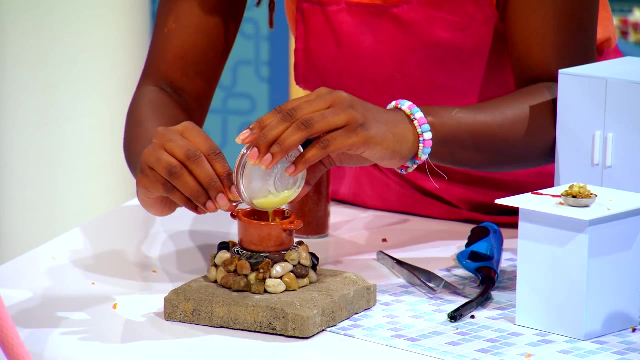 She might. I saw she had a lot of flavors. I feel like in this round the competition might be a little tough to beat. I need to make sure that all the vegetables are cooked all the way through, because I don't want the judges to be eating raw vegetables. 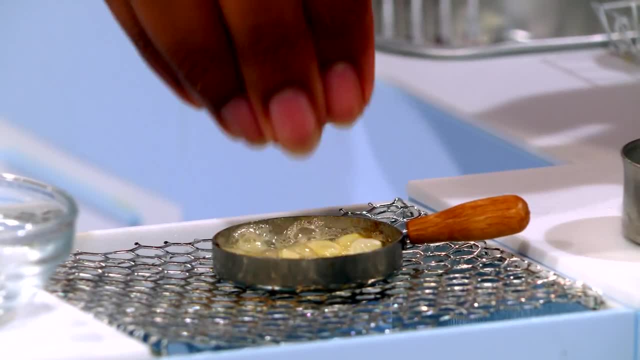 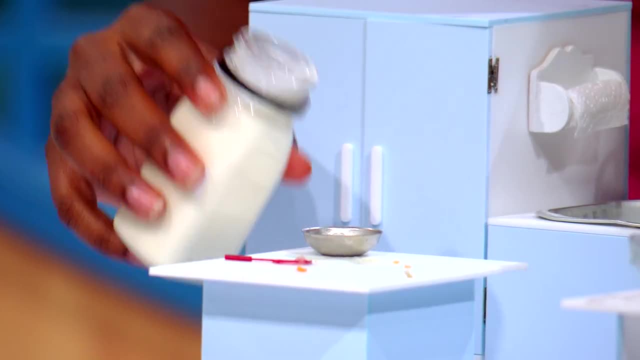 Totally, It smells amazing at this station. It does. So what is your inspiration behind this dish? So my inspiration is roasted corn because, like, when you're camping, you roast things And I actually really like that. I actually really like these corn bowls. 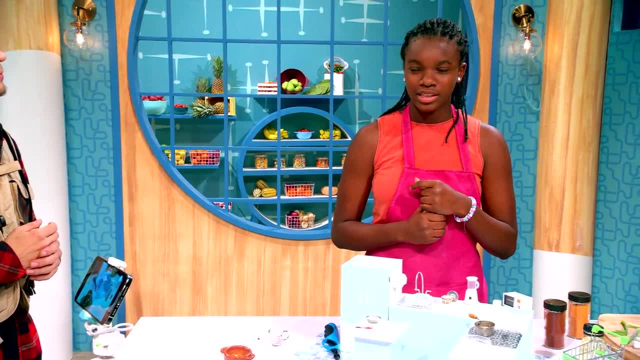 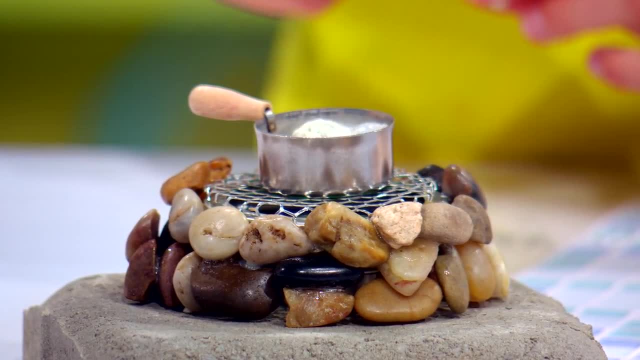 They're from Farmer's Market And it has like corn butter cheese Oof. It's very camping feel Definitely. Gabriel. tell me what you're doing right now. There's some bubbling going on here, Yep. 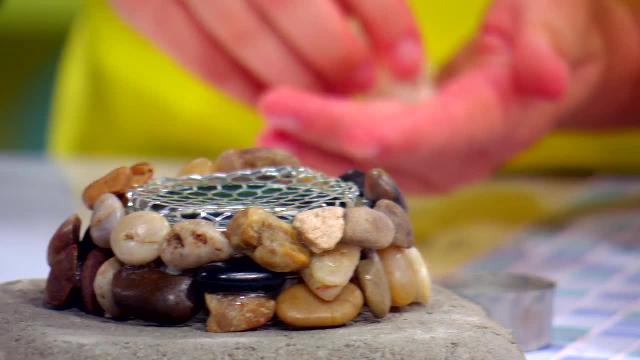 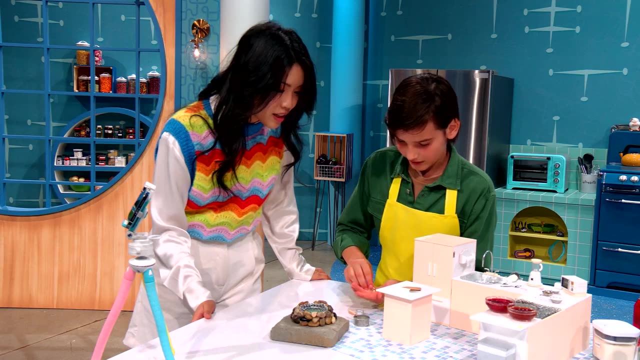 That's actually not too good. The sauce was bubbling, And you really don't want the sauce to bubble because it might mean that it's going to get burnt. What is in there Is that dill. That's dill with heavy cream and Parmesan. 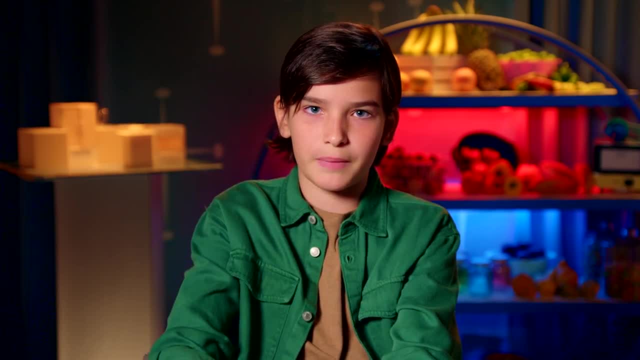 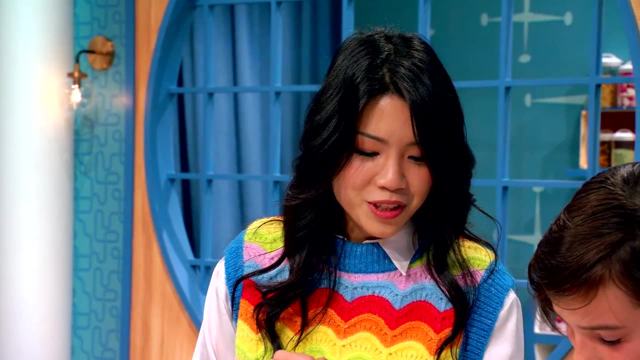 So I was just like putting it on the stove, mixing it until it bubbled, then taking it off, still mixing it and repeat that, And then I still got my sauce. So that's nice. I know there's only a little bit, but I can smell it. 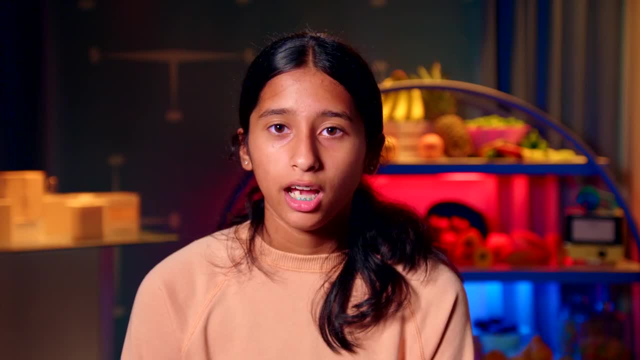 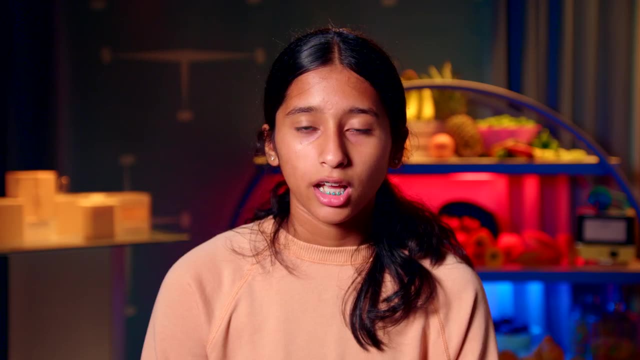 It smells really good. I have to cut a little toothpick And then next I have to stick those red onion, green bell pepper chicken that I put spices on on toothpick, And then I'm going to grill it over my campfire. 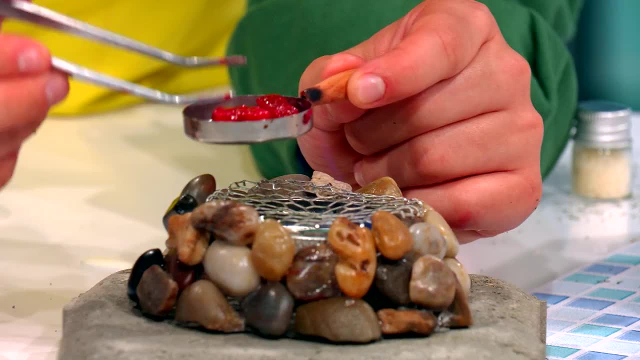 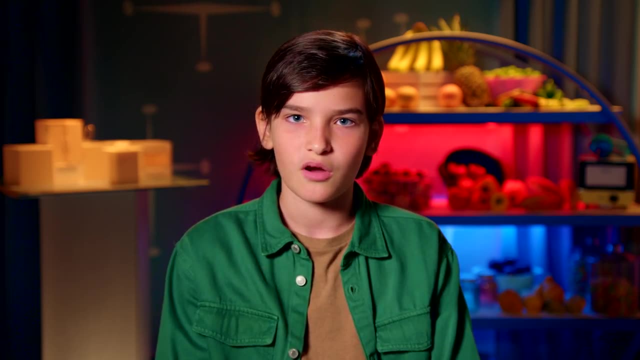 I'll need to be cooking the salmon correctly. I want all sides to be pretty much looking the same. If one side burns, that's going to be horrible, because that burn you're going to taste that throughout the salmon because of how small it is. 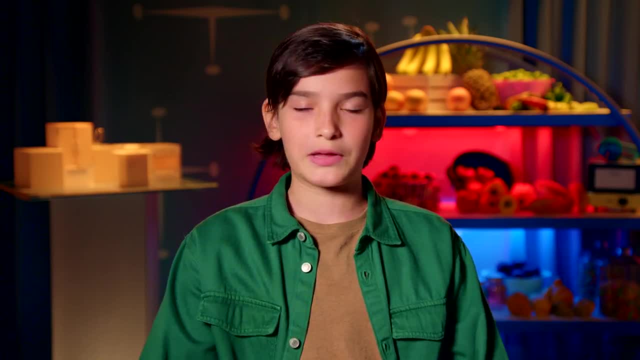 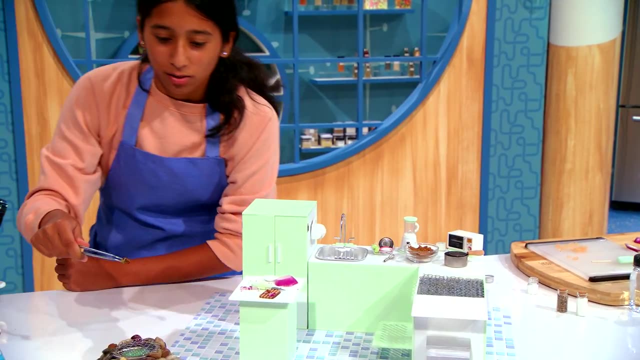 Hopefully the judges will like my dish. Hopefully the hamsters- oh my gosh- they will come after me if I don't do good. So I'm fighting for my life here, you know. So I'm putting it on, but not putting it on here because I don't want it to burn. 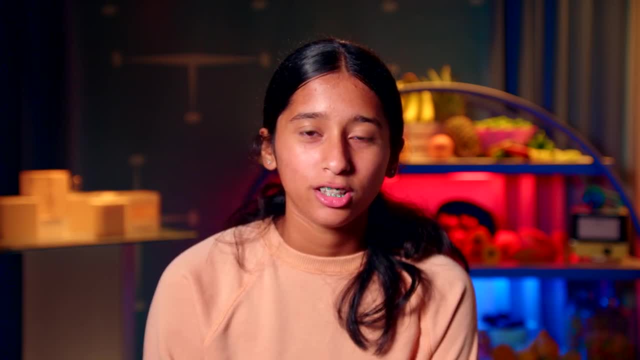 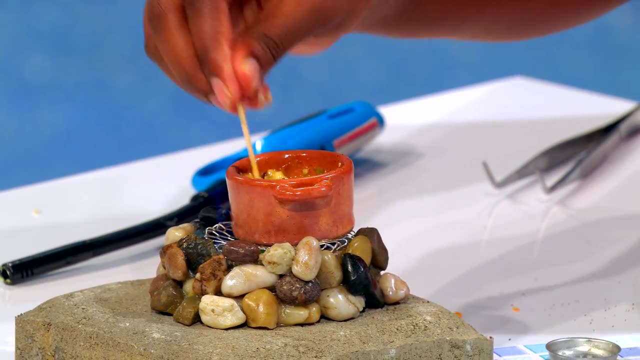 My favorite tiny food tool to use is the tweezers, because it makes things easier to put in the oven without burning myself. Now I'm adding heavy cream just to make sure that it's creamy enough. Two minutes left, everybody, Two minutes. 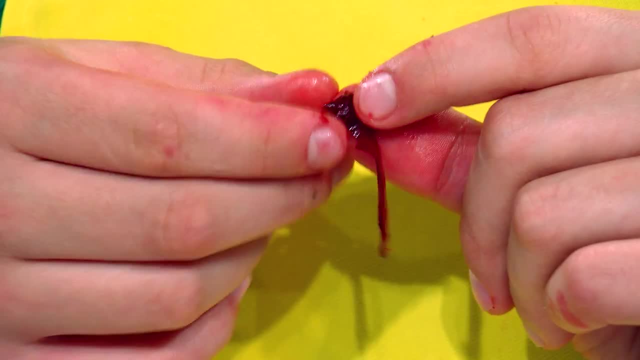 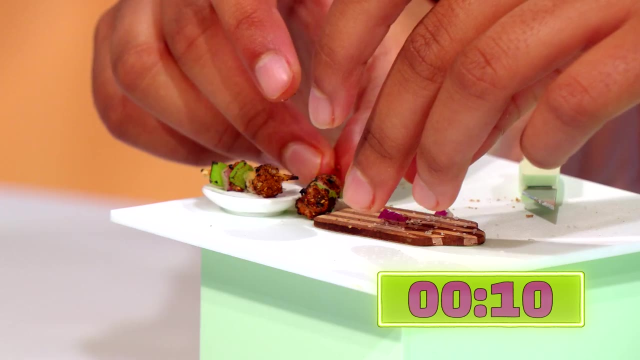 So curling the rows. I've done this before, but, like now, making it even tinier, it might be somewhat difficult. All right, chefs, count it down with me: Ten, Nine, Eight, Seven, Six, Five. 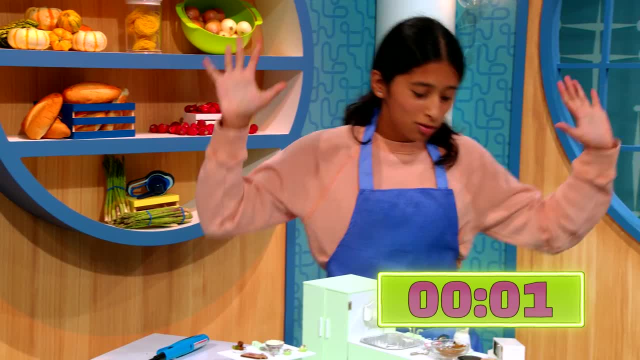 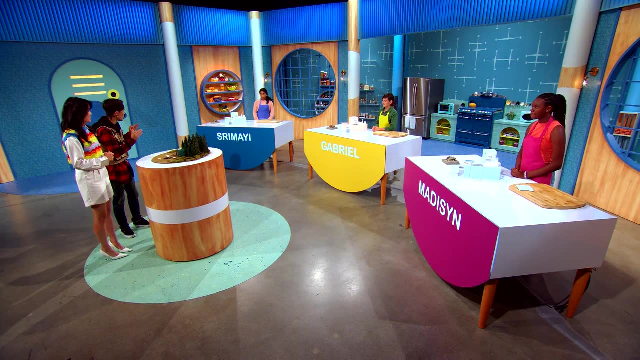 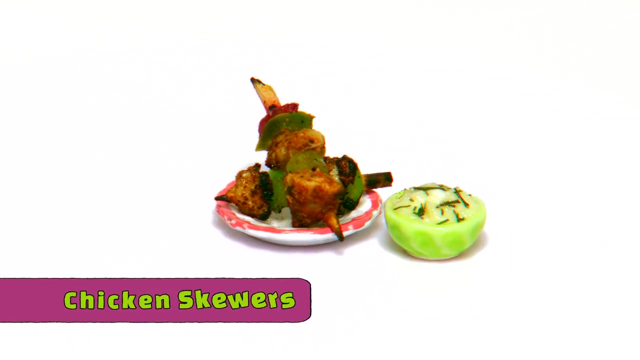 Four, Three, Two, One, And that's it everybody. Great job, everybody, Great job, Great job. All right guys, this is the moment of truth. Shamai, let's see your tiny dish. Wow, So gorgeous. 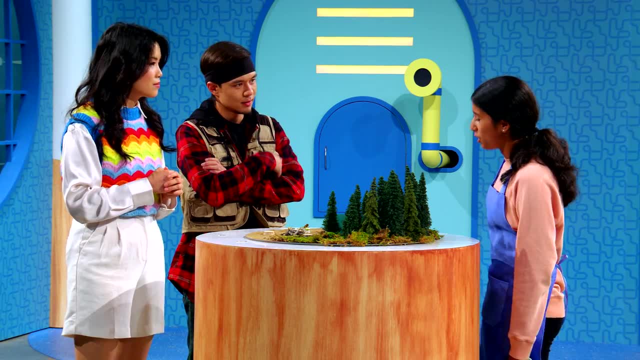 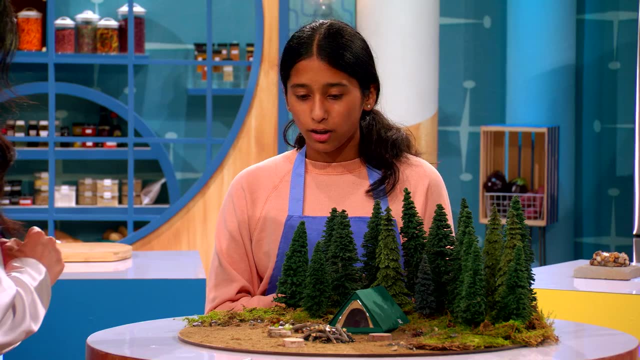 Tell us about this dish, These chicken skewers. they're inspired by my dad, Mm-hmm, And I put bell pepper and red onion. The dip, again, was Sour cream, mayo and dill weed. I don't know what to say. 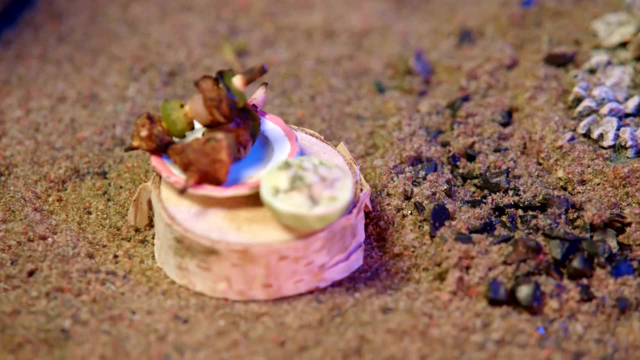 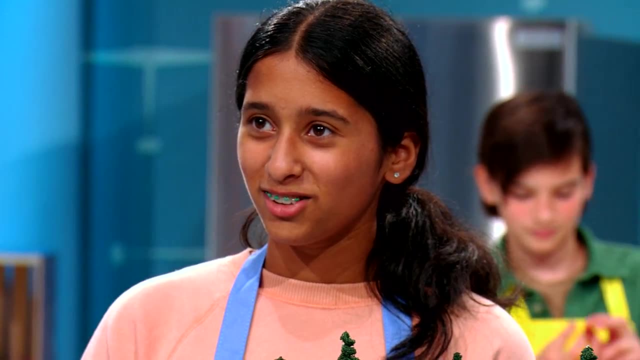 I mean these kebabs. they look like kebabs, just tiny. I'm just so wowed by how you're able to get each piece almost like identical in size, because that's like a big thing about skewers. 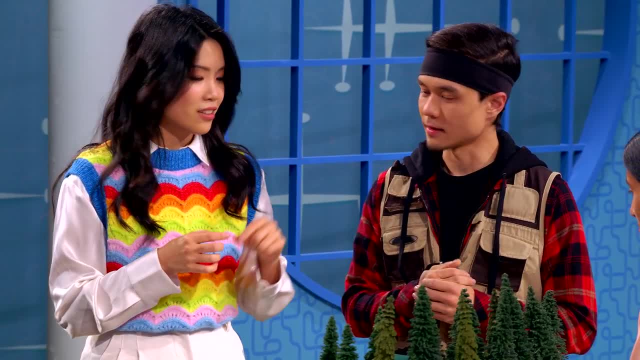 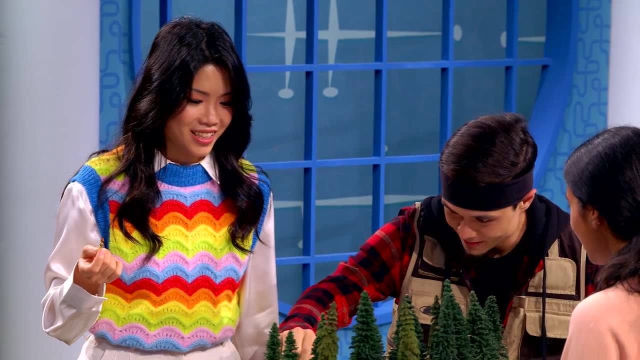 You want them to be equally portioned out? Yes, All right, I think it's time for us to get a little taste. Oh my God, All right, I'll go for the dip. Two skewers for two people. Two skewers for two people. 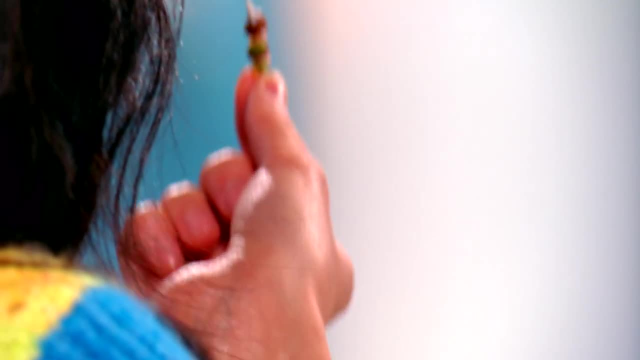 I appreciate it very much. Beautiful Cheers, Cheers. Oh wow. How does this tiny food have such big flavor? I cannot get over it. Right In that tiny bite there's so much like. there's like the red onion and the green. 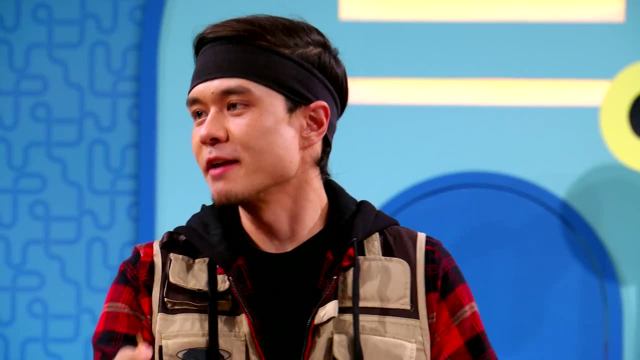 pepper and the chicken and the spices. It's like you get all of that at once. That's not something you can normally have. I love the way you kind of measured everything out so that everything is almost equal, and that's why I love it. 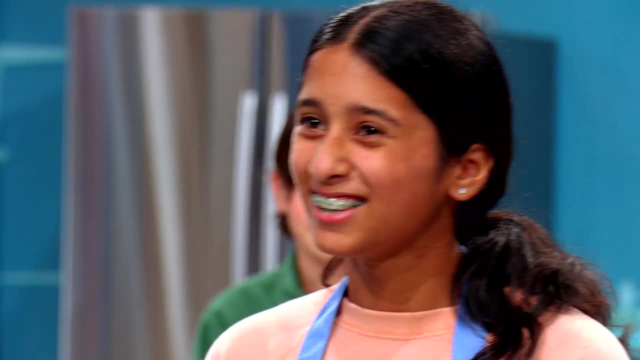 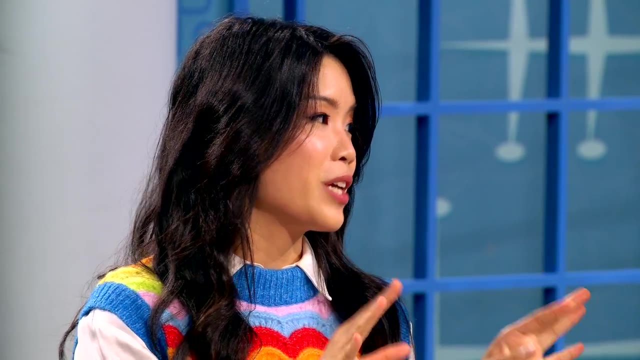 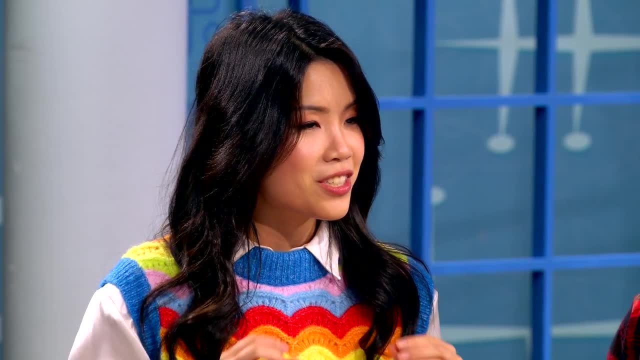 I don't even want to taste it, Unless you bring everything out so that everything is almost equal, and that's why everything just ties in together. Oh, wow, Bro. it's so weird …I'm still experiencing the flavors in my mouth. 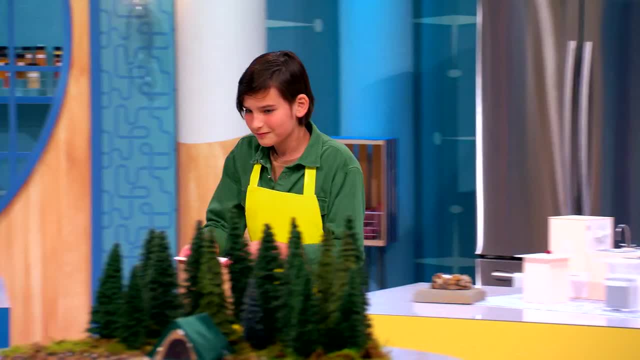 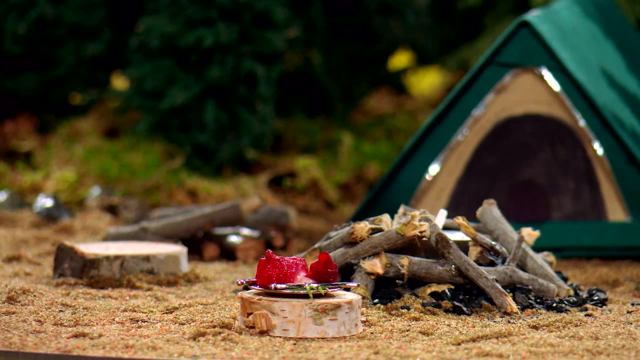 I don't want it to end, Bro. it's so weird. Thank you, Thank you. All right, Gabriel, come on up Show us what you got. Look at that Man…. Ooh, it's so tiny, It's so delicate, that rose. What is the name of this dish? Rosa salmon, Rosa salmon… Okay, fancy, Tell us what we have here on this plate. All right, So you have your salmon marinated in orange juice, juice, beet juice, soy sauce, salt pepper, sugar, the usual. 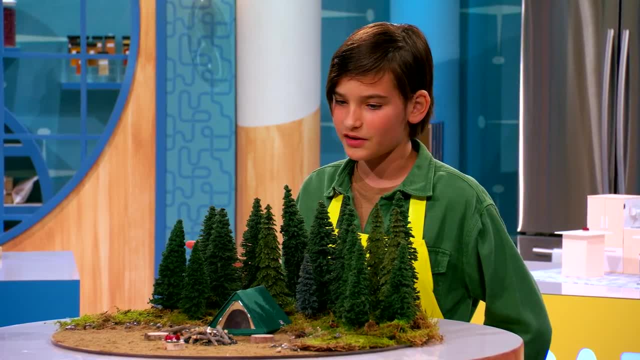 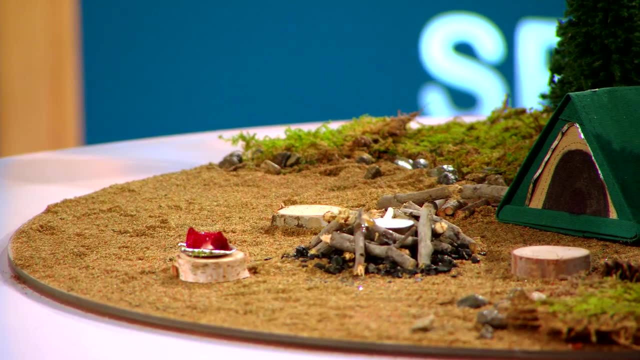 On the left, that's the rose That's marinated in the same things, only with vinegar, red vinegar. The sauce, that's heavy cream with some dill, And there's also a glaze on top of the salmon made with the marinade that it was marinating. 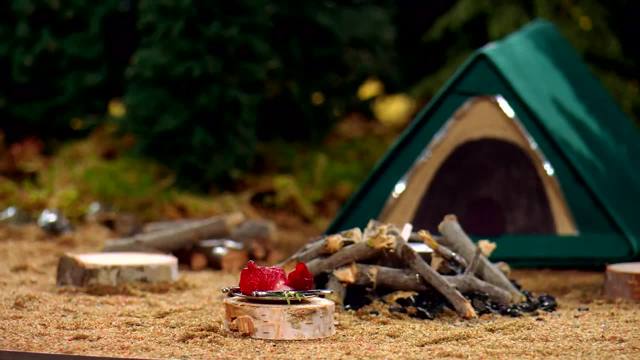 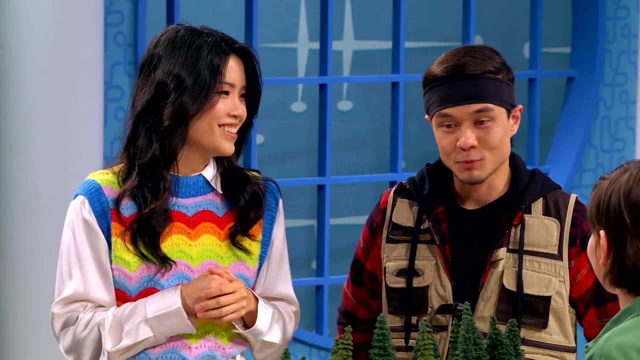 in with a bit more sugar. Ooh, OK, There are many layers to this dish. Yeah, You really know how to camp in style. Got to ring everything. This is what they call a glamping nowadays. Why sacrifice This? looks so good? 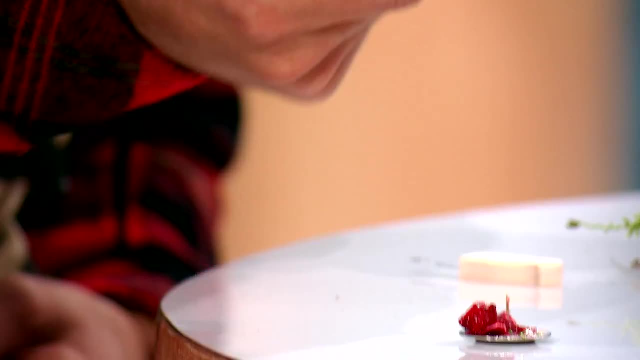 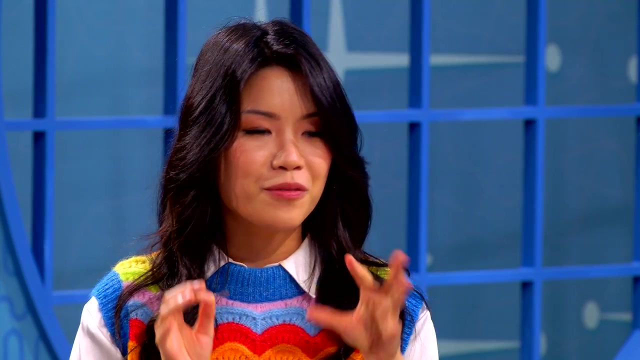 I'm going to go for the salmon first and then the rose. Get a little of the sauce. Beautiful color, Oh wow. I love the freshness of the beet and the texture of the fish. Yeah, 100%, I'm going to dig into this rose. 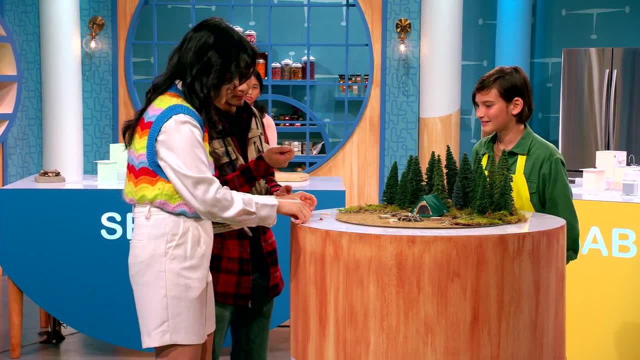 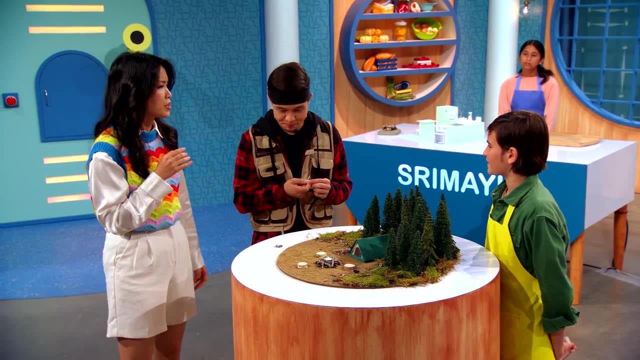 OK, There we go, There we go. All right, go for it. Yeah, I'm liking the bitterness. I mean, proportionally It's a very small portion. Yeah, it might be because there's a lot of sauce on it. 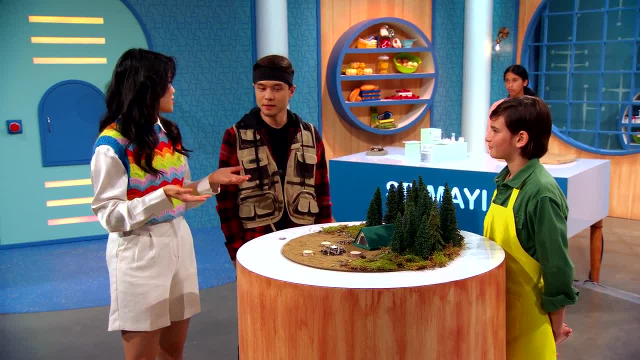 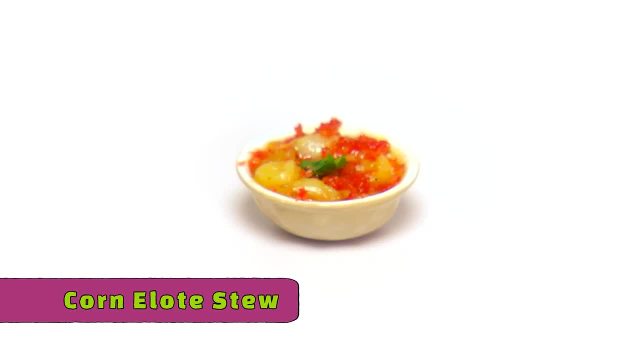 True, true. I love it when people make edible decorations, because you can eat the entire thing. You should be really proud of yourself. Thank you, Madison. Last but not least, So, what is this? So, this is corn elote stew. 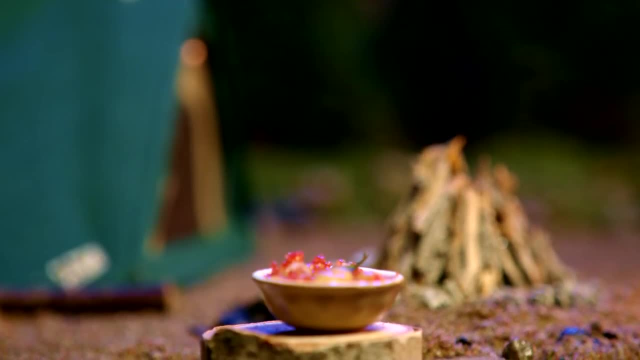 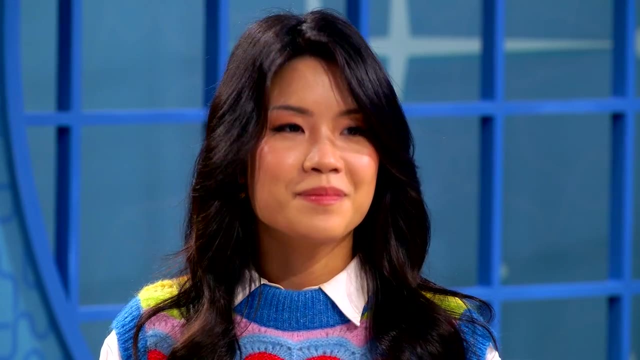 It's based on corn elote, which is like corn butter and there's like different stuff on it And I really like roasted corn, so that gives it like a better flavor, like with the butter. That's why it smelled really good over there. 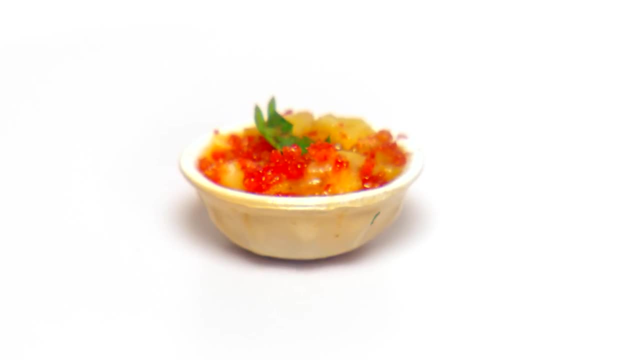 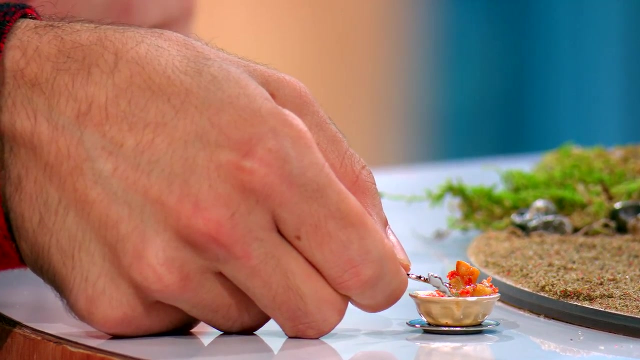 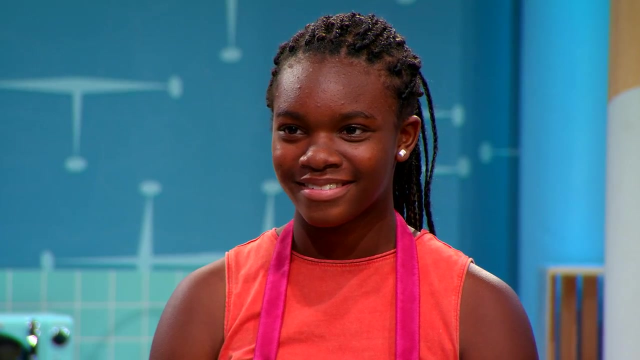 And then I finished it off with some cheese cilantro and cheese dust. So when can we dig in, Please? I can't wait any longer. Go for it. Go for it. Challenge, All right, well cheers, Oh my god. 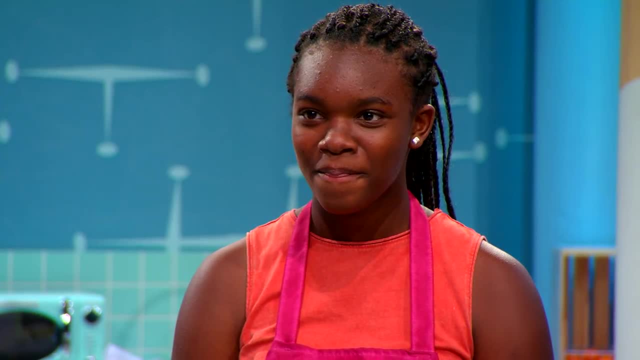 It is creamy, It is spicy Like it's very slight, but you do get a little bit of that kick. I could taste the cheese, the potatoes, the corn For a stew. you got the consistency, You're right.